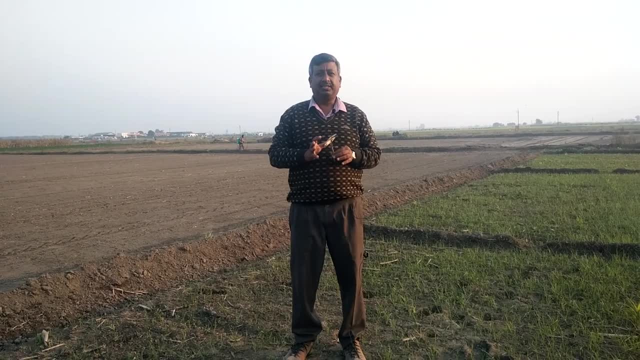 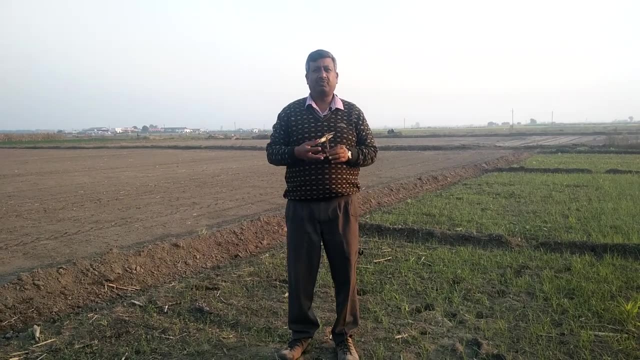 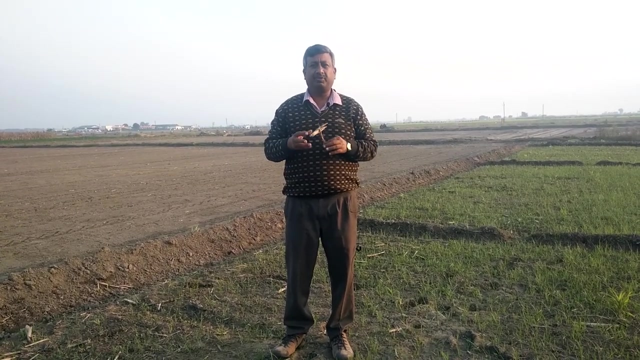 there is very rapid, very fast decomposition And then crude protein. it takes time, further time taken by hemicellulose, then cellulose, fat wax and the most resistant material, or which take very more time for decomposition. So this is the first step, Then the second. 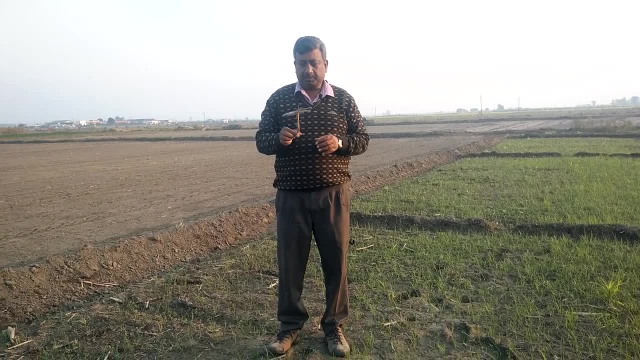 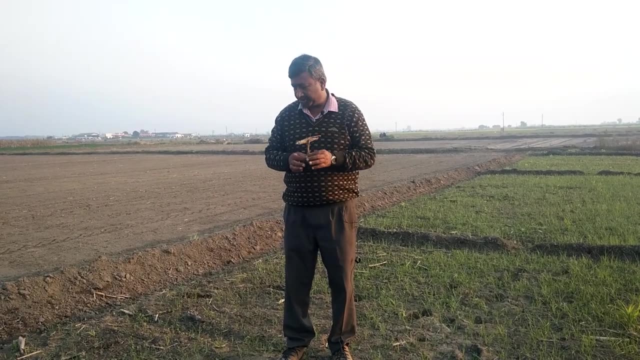 step is very difficult, dein z immer lang lang וח frança Chapel. The third step is decomposition and the most two necessary important step is decomposition. The second step is decomposition and very slow decomposition by lignin. So in this Kosher. 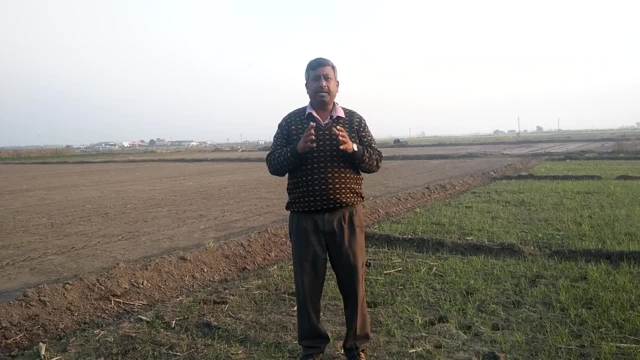 gene chromosome. if there is simple protein or sugar or starch then its decomposition becomes very fast, means it will quickly go rot easily. We mean decomposition by rotting here. If it contains lignin then its decomposition will be very slow, And woody plants generally. 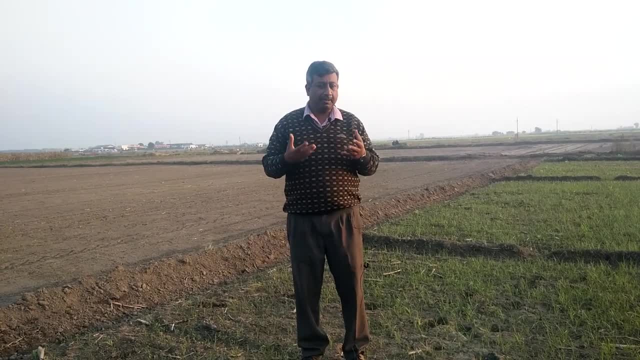 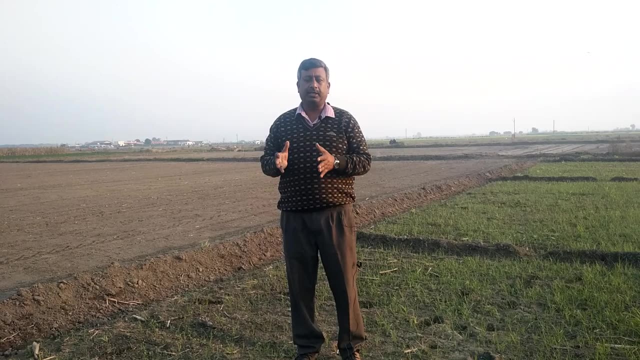 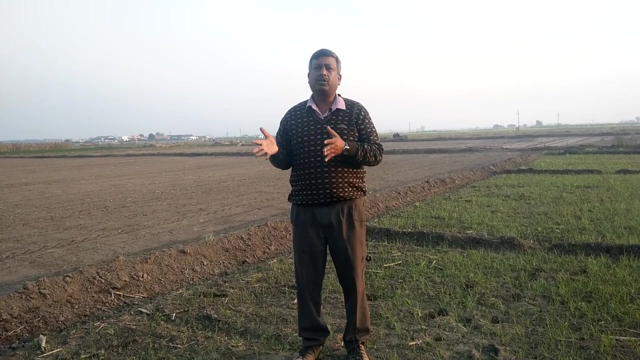 contain lignin material. That is why decomposition is very slow. So this will depend on what perd drawer that uses. If we cut a tree and put it in the soil, then it will definitely have more cellulose and more lignin, so its decomposition will be slow. 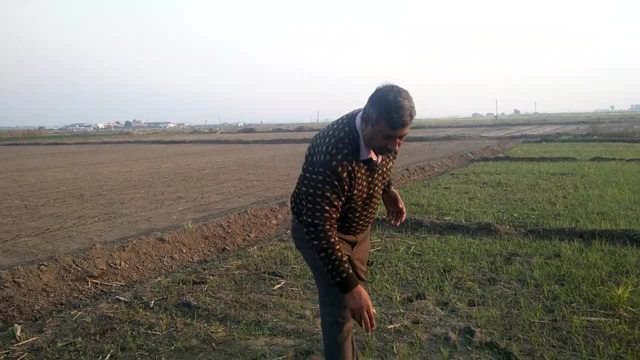 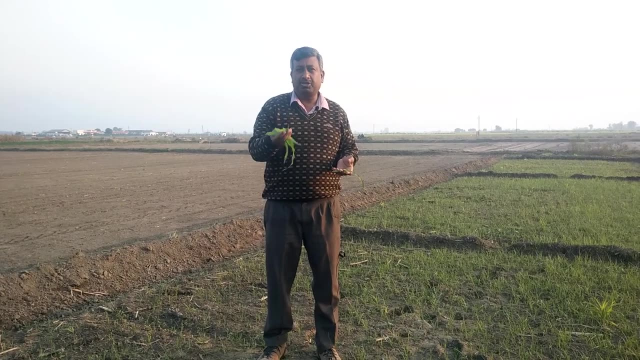 And if it is a very succulent material like these leaves? see, it is very succulent material. no cellulose or haemicellulose has been made in it. there will be simple sugars or simple proteins, and when we put it in the soil and decompose it, then what will happen? it will 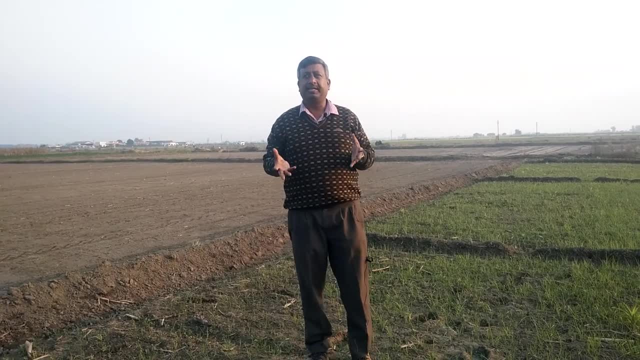 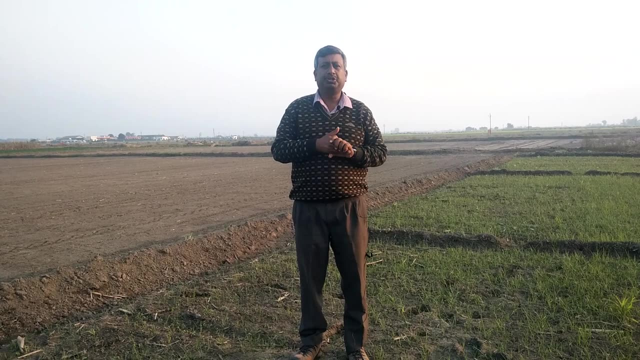 decompose easily. So it will depend on what type of material it is. so where will be the very fast decomposition? it will be in sugar or starch and it will be in simple proteins. so I told you one series how the rate of decomposition is getting slow. I will tell you that series again: the fastest. will be sugars, starch and simple proteins. then crude protein- it takes more time- then haemicellulose cellulose, then fat and wax and in last lignin. So if there is a lot of lignin, a lot of cellulose, then the decomposition will be very slow. 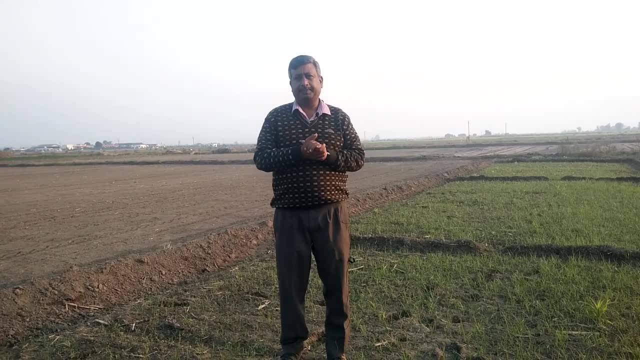 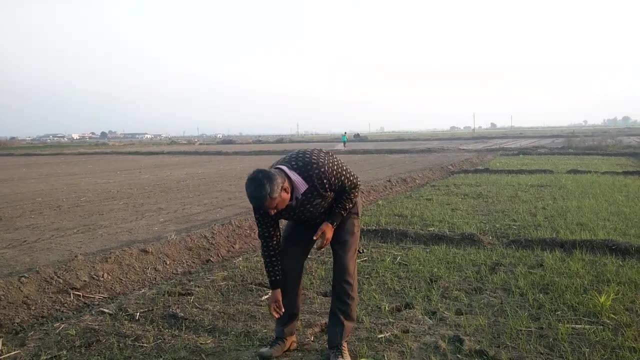 so I told you this now how this decomposition happens. this is very important: how this decomposition takes place. actually, several microbes are present in this soil. this soil has a lot of microbes. there are a lot of microbes, and assume that if we take approximately one, 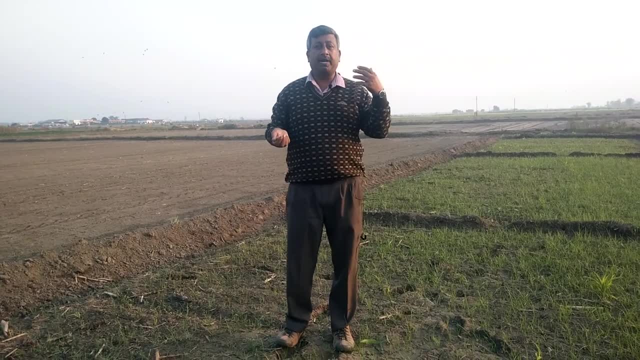 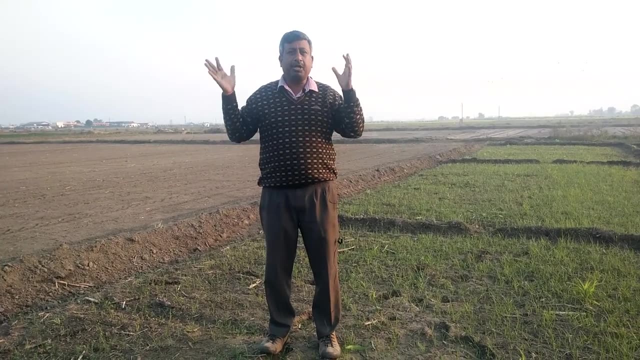 gram of soil. in one gram of soil there are about one crore microbes. one crore microbes can be in it. so you can assume that how many microbes will be in such a big field and these microbes will be there. So the first one is the secretes enzyme, several enzymes, very common enzyme is urease. 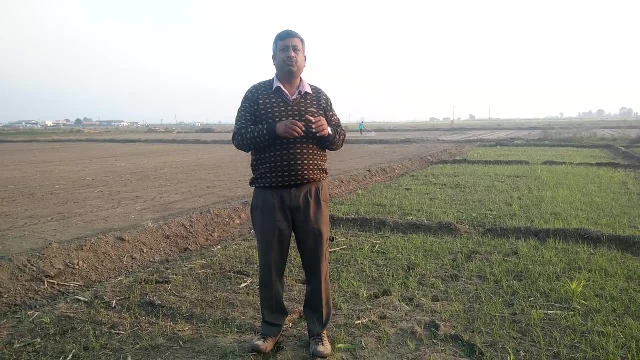 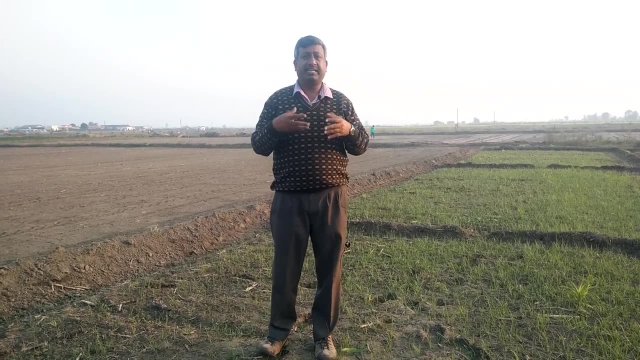 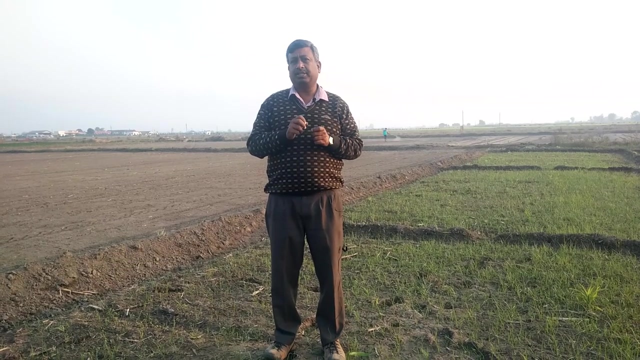 urease enzyme. urea is known as urease enzyme, urease, then protease enzyme, phosphatase enzyme, amylase, sulfatase, all these enzymes- there are number of enzymes- are secreted by microbes and these enzymes, these enzymes, break down the complex organic material in 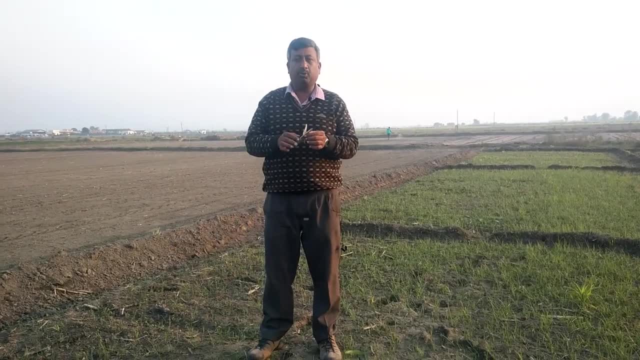 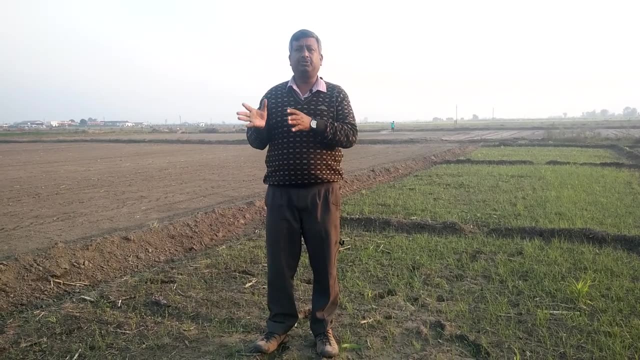 these residues. so in these residues, the material which is in it, cellulose, haemicellulose. what will be the breakdown of it? it will be from the enzyme and the carbon in it. that carbon is utilised by microbes for their cell synthesis, so the microbes will do the bacteria. 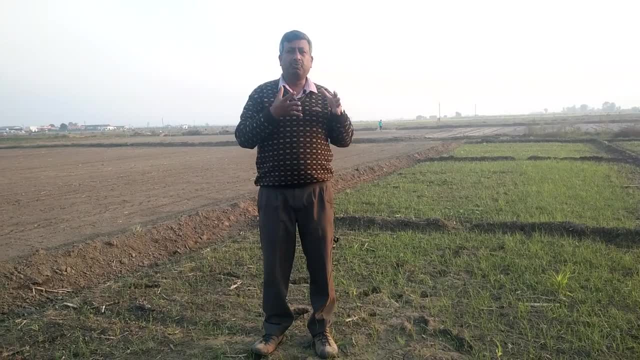 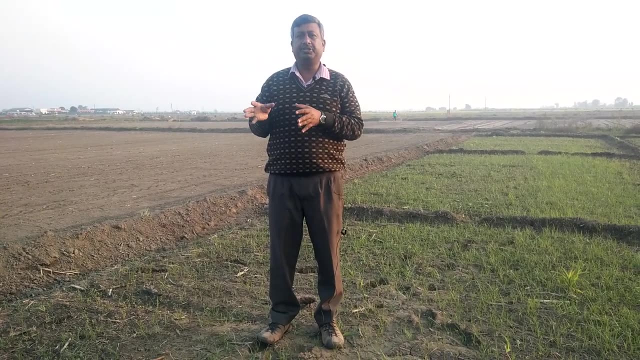 which will do the synthesis. they will do the carbon from it, and carbon is food source. actually, carbon is food source. so that's why they attack this organic material or residue, plant residue for the carbon, for energy source. so when they will take it for energy, they 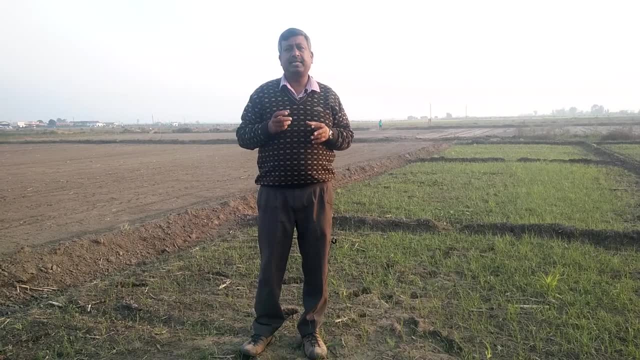 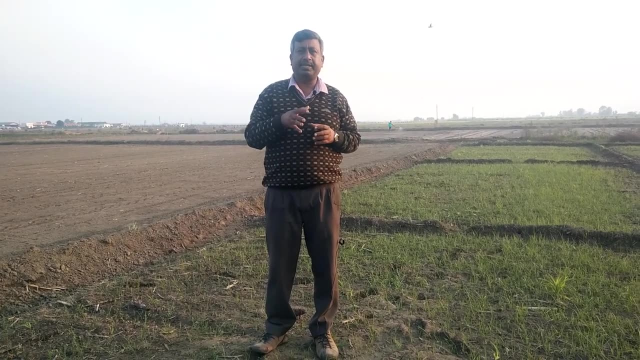 will attack the carbon. so what will they do? they will use the carbon in which the cell is. so because of the carbon, their microbial population will increase. when the population increase, then they will further attack. then enzymes will appear. then further attack. then they will use the carbon and then attack. then their population will increase because they are finding carbon continuously. so for the ones with highly oxidisable carbon that is very good food for microbes. so the more oxidisable carbon will be so their cell synthesis. 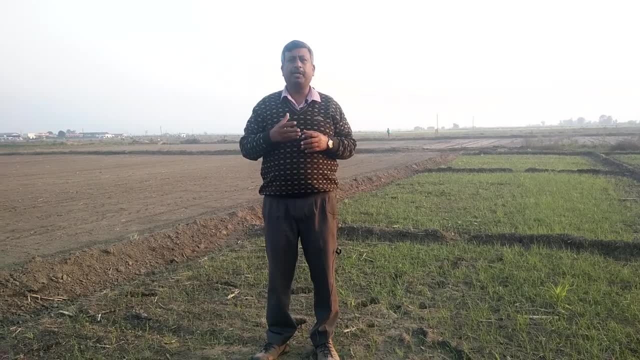 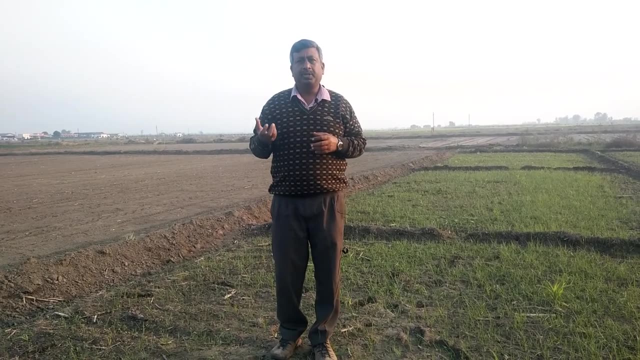 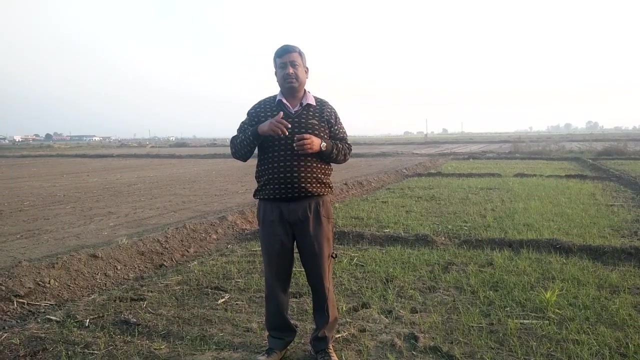 will be added, so their population will increase. similarly, when their population will increase and their respiration will increase, so CO2 rate will also increase immediately in the form of CO2.. CEOs, Now, during the this decomposition, actually carbon is used for cell synthesis and simultaneously, 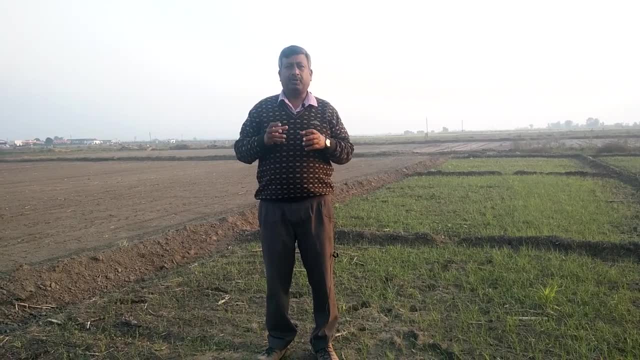 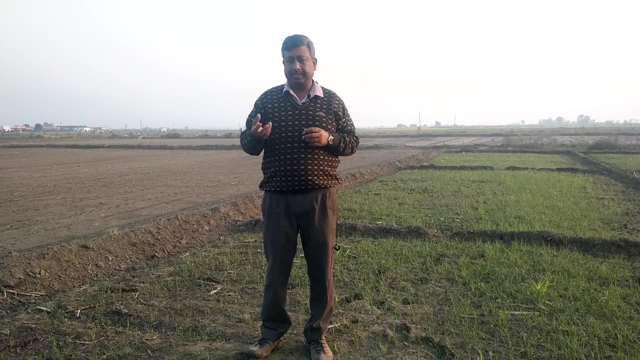 there is synthesis of protoplasm inside the body and for the synthesis of protoplasm nitrogen is required. that's why they drive the nitrogen and other nutrients are also required by microbes like phosphorus. they drive the sorry phosphorus, calcium, magnesium, other nutrients, the microbes. 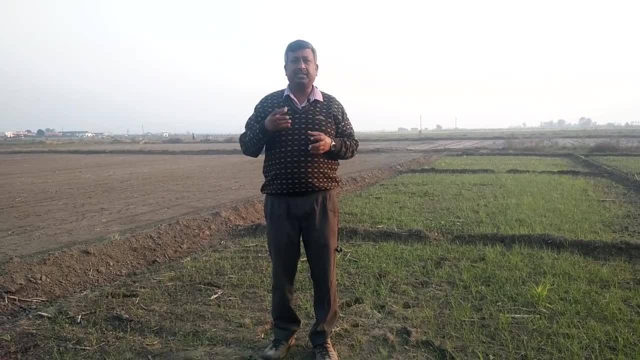 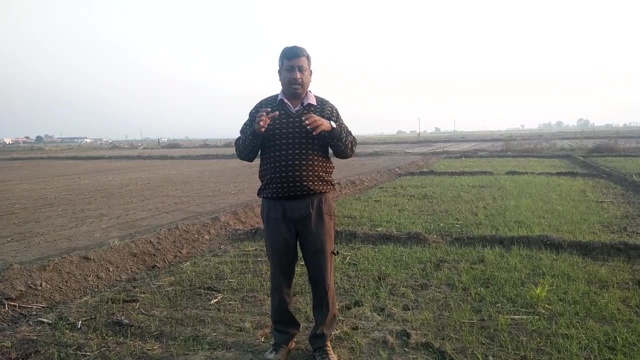 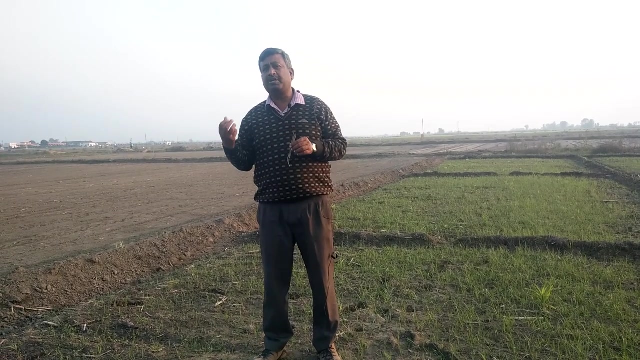 need these nutrients also. that's why, during the decomposition, these nutrients are taken by microbes and retain these nutrients in their body. so now, the nutrients which were in this, which were in these residues, which were supposed to come in the soil of the decomposed, they went to the body of the microbes, because who needs it? microbes need it, and this process 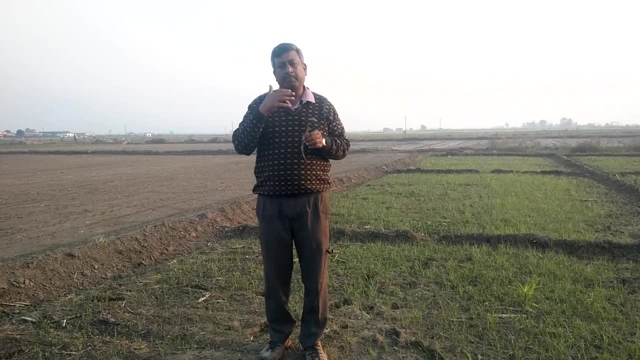 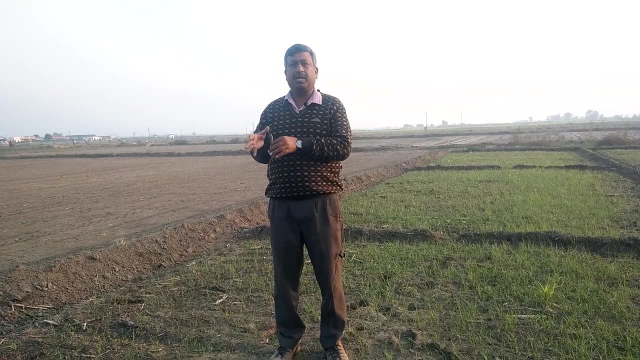 is known as immobilization. so as soon as decomposition happens, immobilization will also happen. definitely, this has to happen. this immobilization process cannot stop, why, as soon as oxidizable carbon is found, carbon source is found, food source is found, microbes are attacked, fungus is attacked, bacteria is attacked, their cell synthesis is done, population. 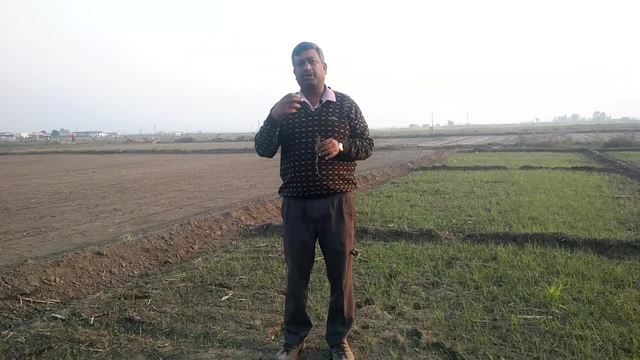 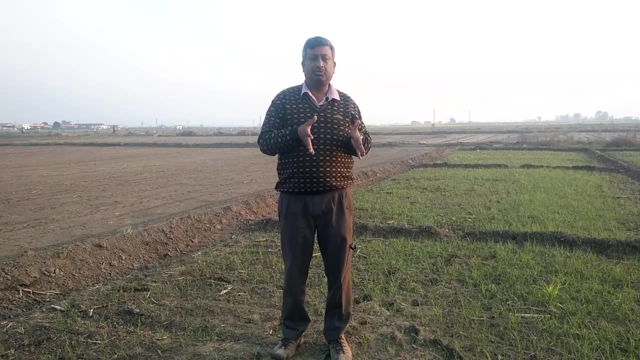 is increased, by increasing the population, what will happen? they need these nutrients and these nutrients have gone into their body for cell synthesis, and this is known as immobilization. so now, what will happen? nutrients are not available in soil solution. that's why not available to plant now, after. 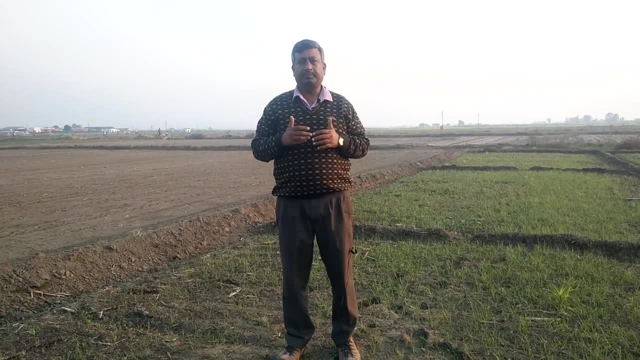 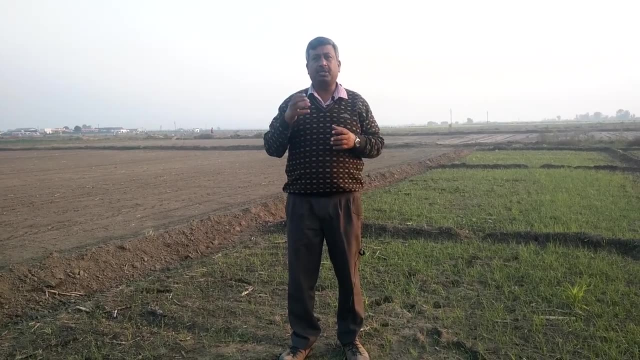 this. what will happen as soon as oxidizable carbon, means the one which easily breaks down, is exhausted? now what will happen? the microbes are very much so. they started taking carbon. what will happen whatever carbon will be there? I read this: residues, whatever carbon will be there in it. 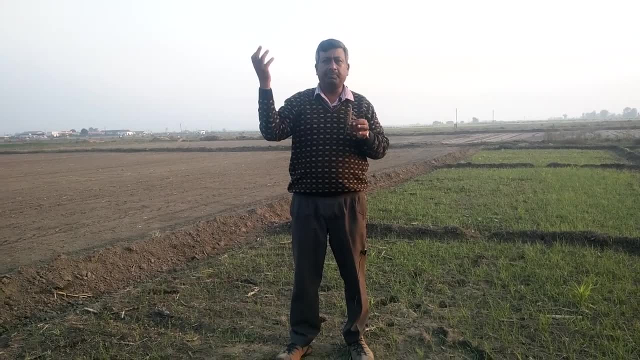 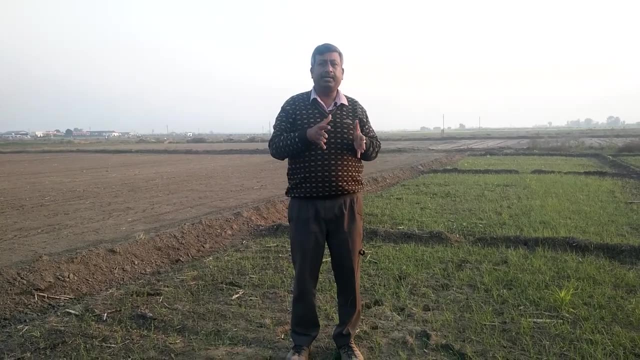 where will that carbon go? it will go to the body of the microbes and it will be emitted through CO2. so when its carbon will be finished, then the population will not increase further. now they will not get food. so what will happen to the microbes? 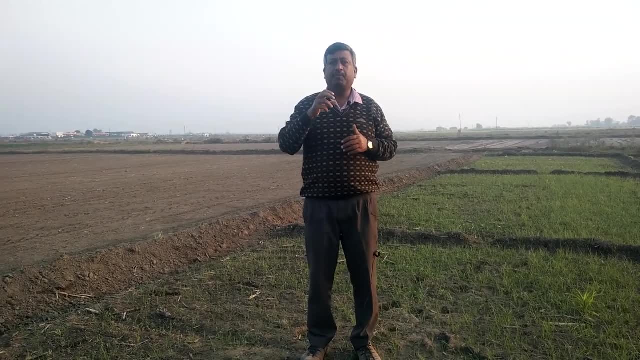 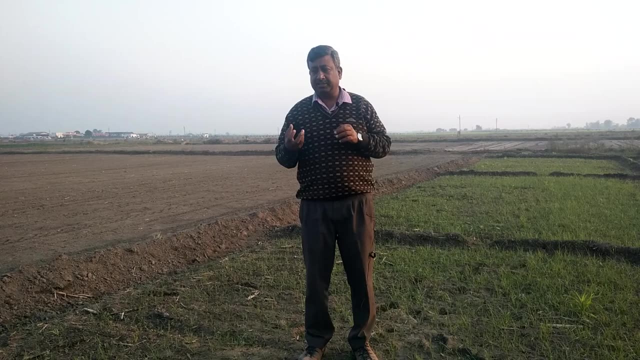 death will happen. so when the microbes will die, then the nutrients which were retained in their body, where will they go? they will come to the soil solution. now these nutrients, whether it is nitrate, phosphate, calcium, magnesium, magnesium, are released into soil solution and available to plant. 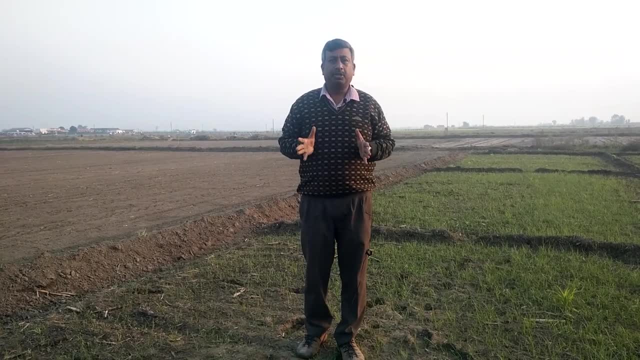 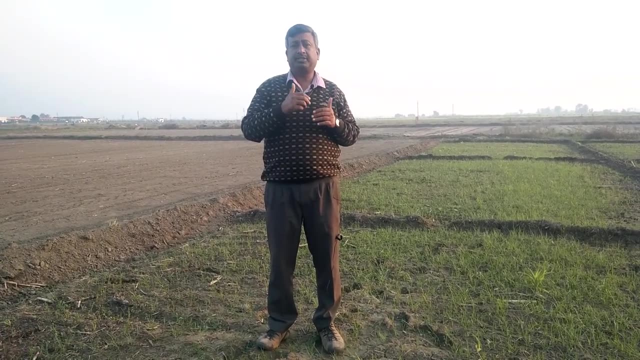 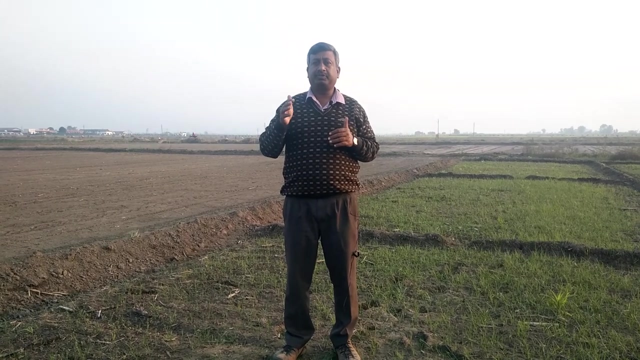 and this process is known as mineralization. so see, both the processes will go. during decomposition, immobilization and mineralization. and immobilization, nutrients are taken by microbes and during the process of mineralization, these nutrients, which were in plant body, are now released into soil solution. this is mineralization. so these two processes will go. now we will. 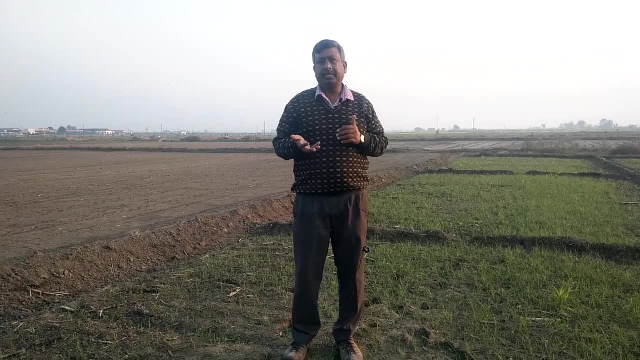 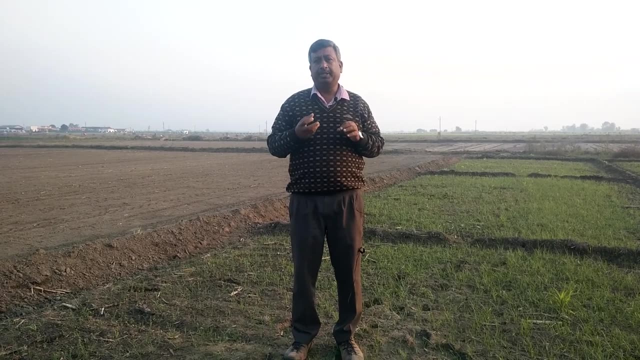 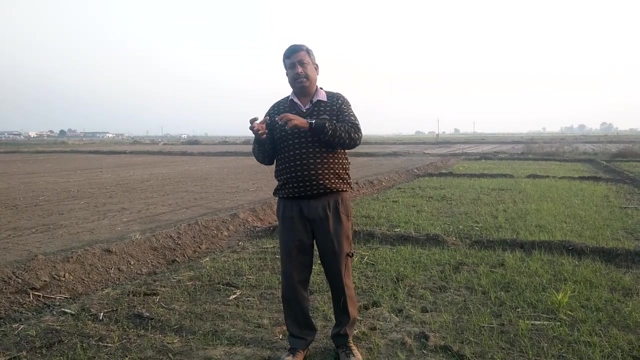 see in the organic and inorganic form, that what is immobilization? from organic form, inorganic form is converted because those which were in organic form in plant residues were in organic form and they are taken by microbes in the form of inorganic ion and retained by microbial body. now in which form did it go? in microbial? 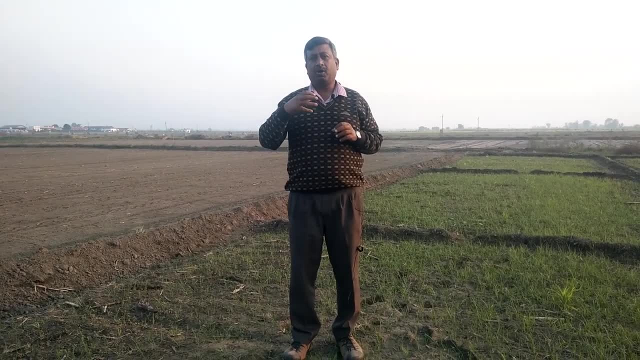 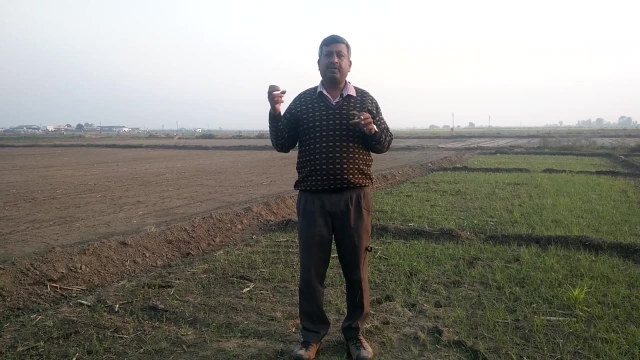 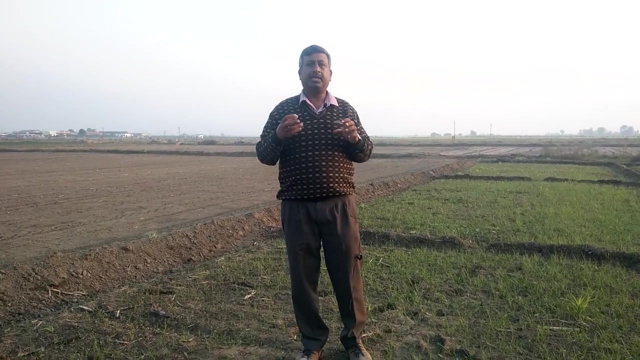 body. again it went into organic form. so those which came from organic form in plant residues form were in inorganic form during the decomposition, Ok, and retained by microbial body, further in organic form. so the inorganic form of soil solution which went into organic form, this is immobilization. so what is immobilization? 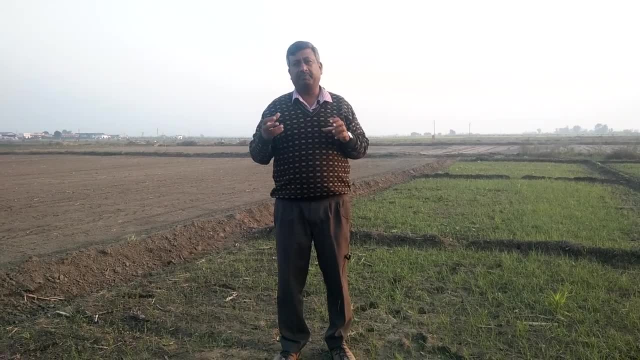 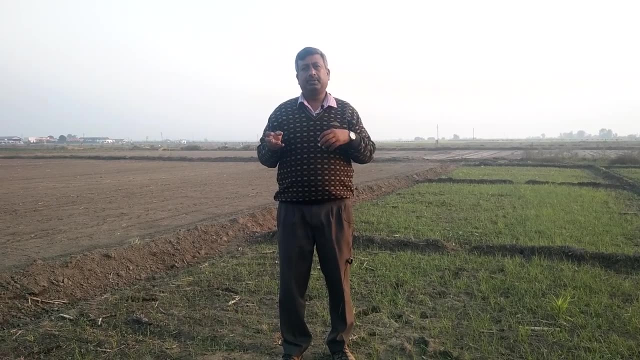 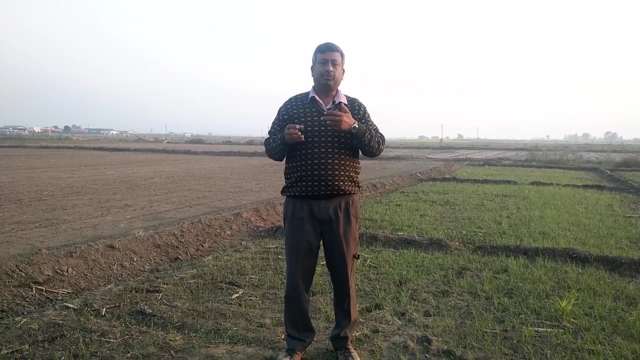 in immobilization, inorganic form is converted into organic form. this organic form is in microbial body and after the death of microbes, nutrients are released from the body. so the body which was in organic form. now how will it come? it will come in inorganic form, like nitrate, sulfate, phosphate, so this will be called mineralization. 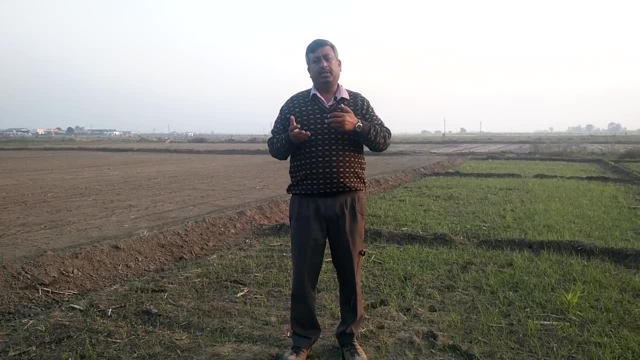 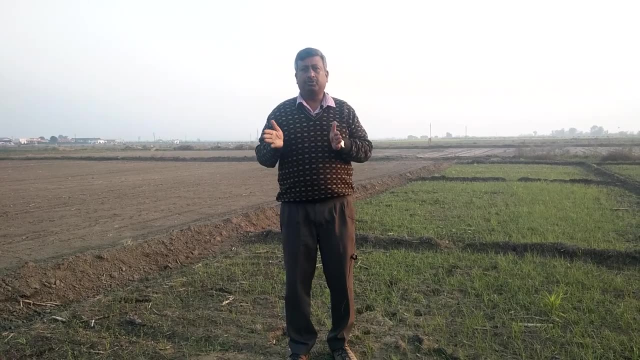 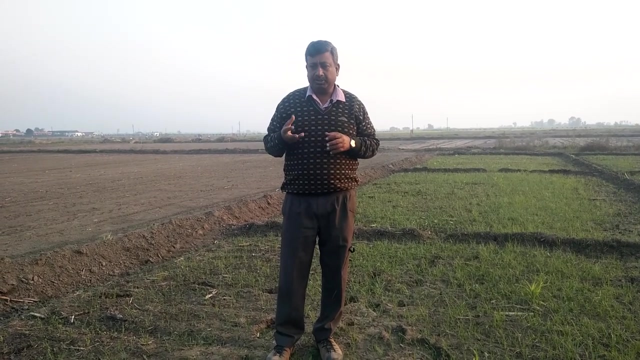 so what will happen? in mineralization, the organic form is converted into inorganic form. so this is the process of mineralization and immobilization. so whenever there is decomposition, there will be mineralization and immobilization. and what will happen? there will be emission of CO2. so this is the process of decomposition. so I have told you. 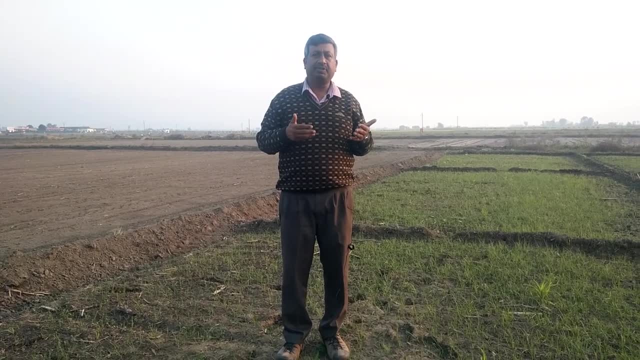 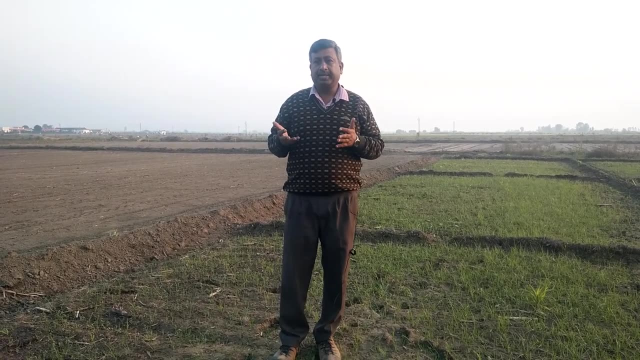 which microbes are involved in this and what is the rate of decomposition? and during the decomposition, what will happen? so see, CO2 will come out, whatever decomposition will happen, and from that water will come out, because whatever organic matter is composed of carbon, hydrogen and oxygen, so carbon will. 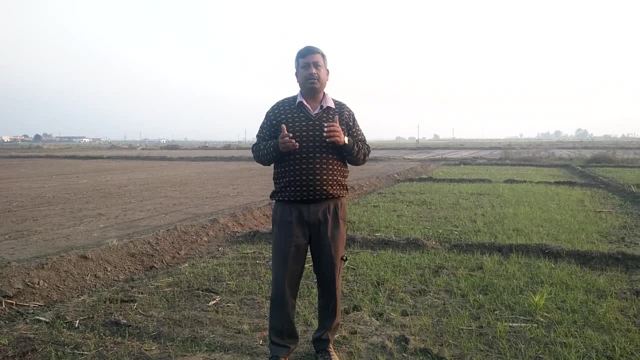 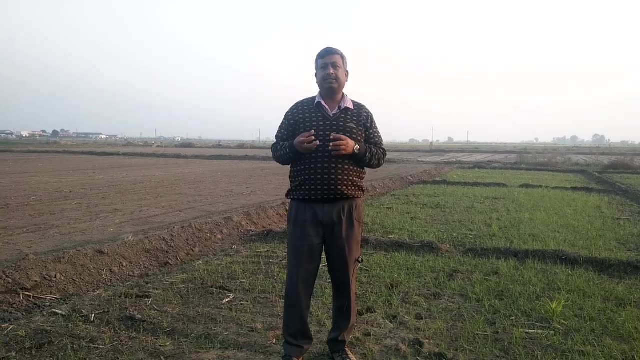 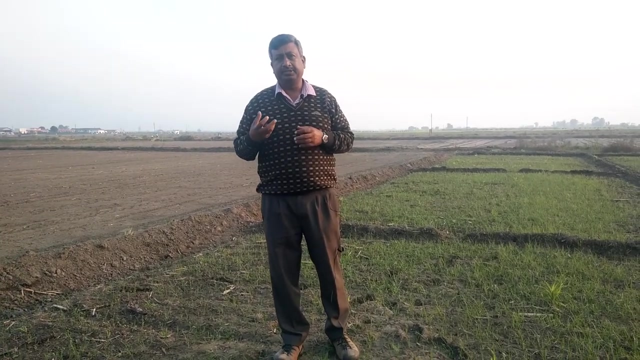 go into CO2 hydrogen, and what will be made out of it? water will be made out of it and energy is released. now this energy is utilized by microbes or liberated as heat. so whenever there is decomposition, heat will come out and energy will be released. so this is a common process. what will happen next? 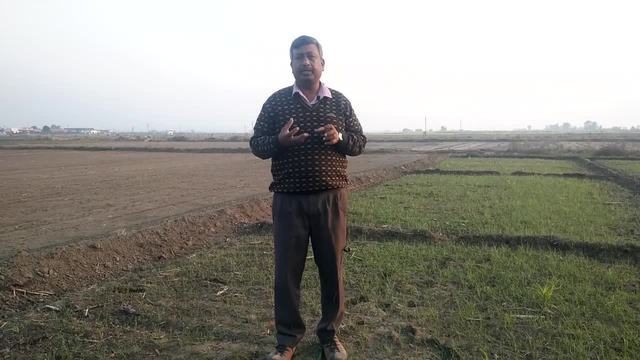 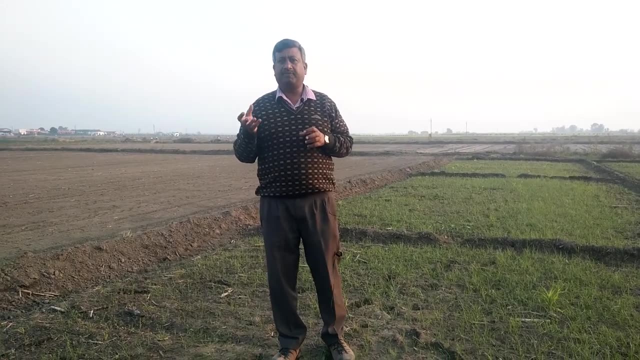 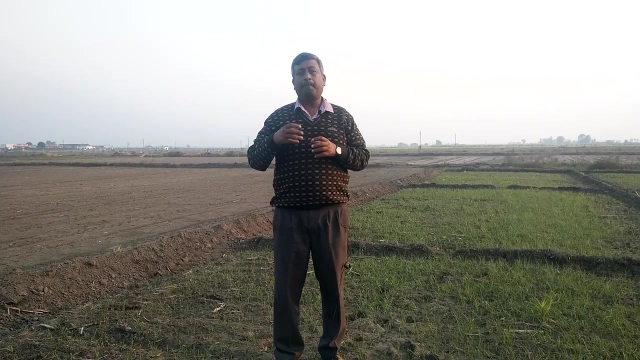 nutrients will be released: nitrate, phosphate, sulfate, calcium, magnesium. this will come out and these nutrients are taken by microbes and further come into soil solution. this will be the second process. third, what will happen? humus formation, which I told you in the previous lecture, that complex resistant material will be made. so the residue that is made will make. 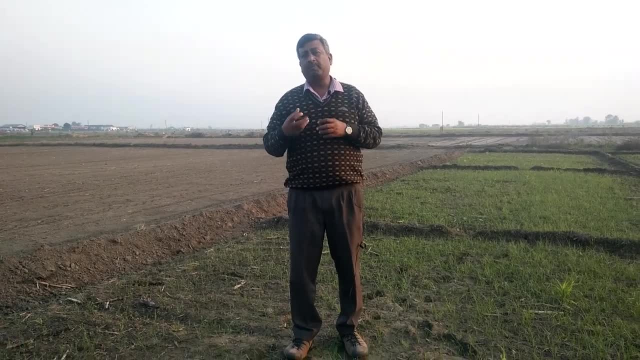 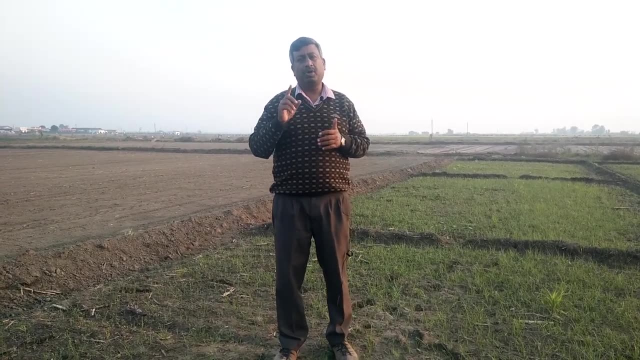 new compounds, new synthesis will be made and then polymerization will happen, so humus formation will happen. so there will be three reactions here when decomposition will happen. number one: CO2- liberation of CO2, water and heat. number second: mineralization of nutrient, mineralization and immobilization. 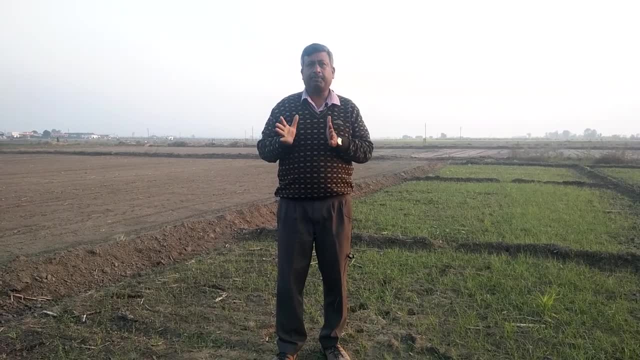 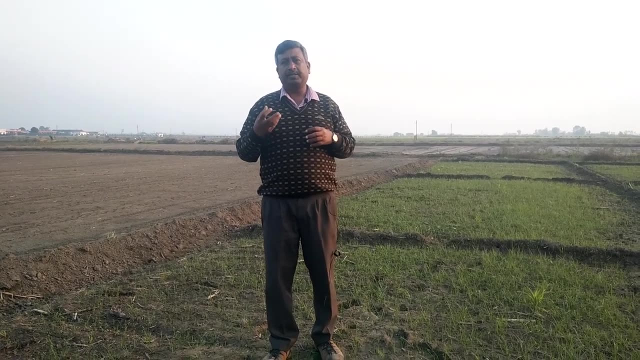 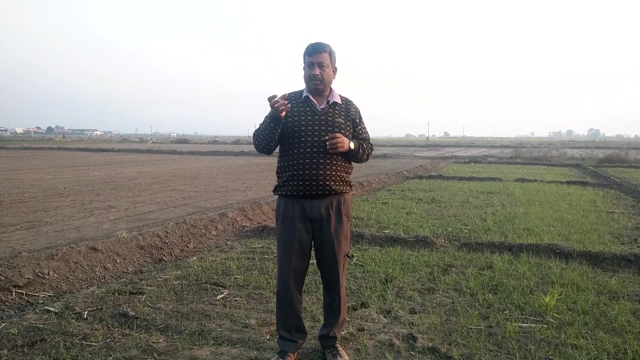 Number third is humus formation. so this process will happen. now see what happens: that the decomposition that was the material, the complex material was in the residue, now converted into simple compound and microbes. attack on this simple compound and these compounds are retained in the body of microbes. and modification of new compounds. synthesis of new compounds. 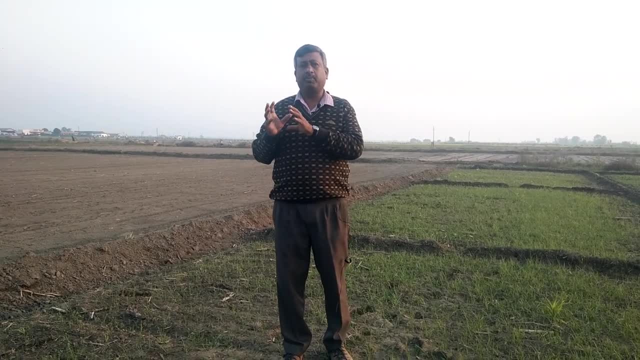 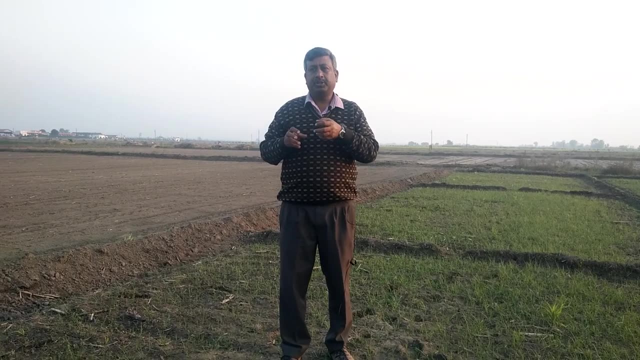 so this modification also happens and new compounds are made in the microbial body. there is synthesis. Now, when the death of the microbes will be there, then we will attack other types of microbes on it and take those nutrients. So where did this happen? 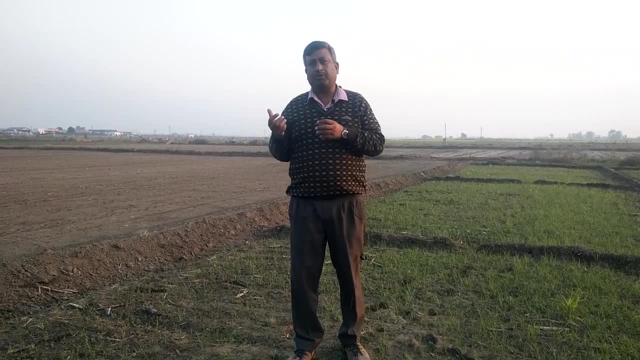 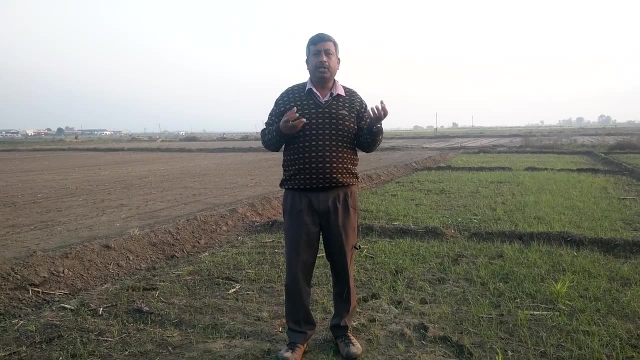 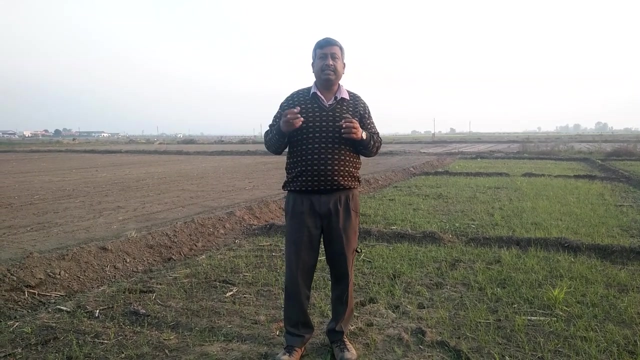 Then there will be further synthesis of compounds in the microbial body. Now, when the death of the second type of microbes will be there, then we will attack other types of microbes on it. So what will happen? in this way? A chain runs and this attack continues until it contains oxidizable carbon easily digestible. 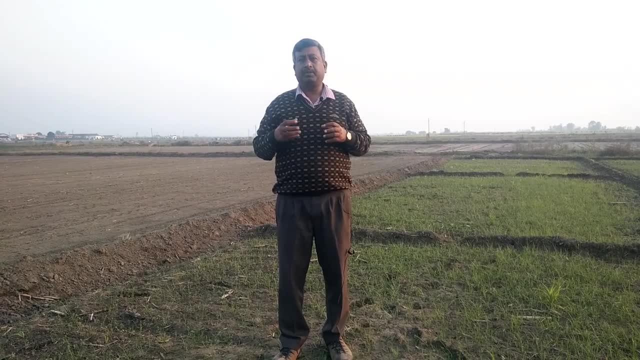 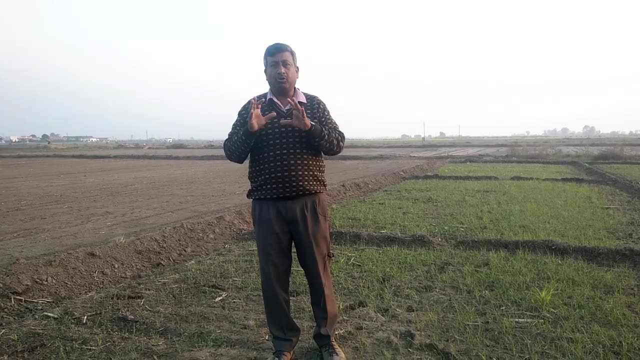 carbon and until the chain remains simple. When the organic compounds chain is very strong, When the organic compounds chain becomes very complex, new compound becomes polymerization. then they can not attack further. This is called resistant material. So resistant material is the material on which micro-subtact is not possible. 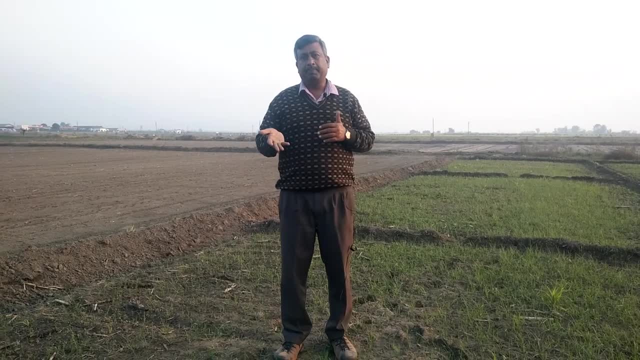 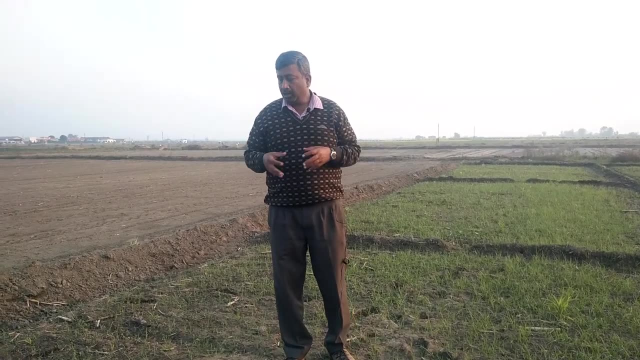 So how this resistant material is made, As I told you, there was a simple breakdown. then new synthesis compounds were made, modification was made, polymerization was done, new compounds were made, complex chain was made and after that it will not decompose further. 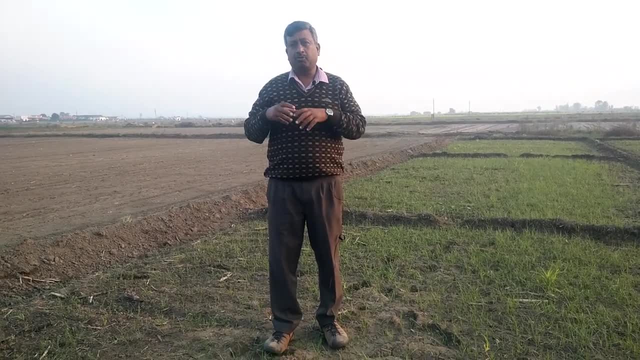 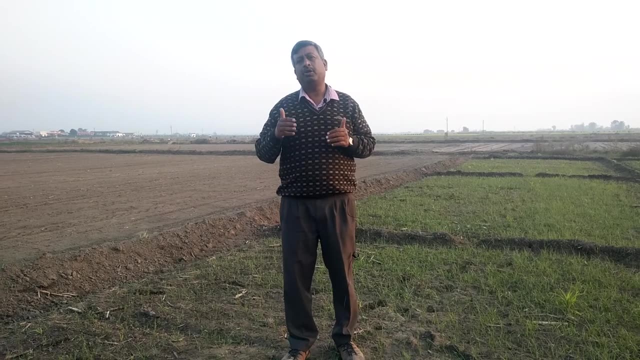 So this complex material became a resistant material. dark to brown color color is given, this is called humus. So this is a process: decomposition will take place. in decomposition, synthesis will take place and polymerization will take place. So humus is made in this way. I have already told you in the first lecture. 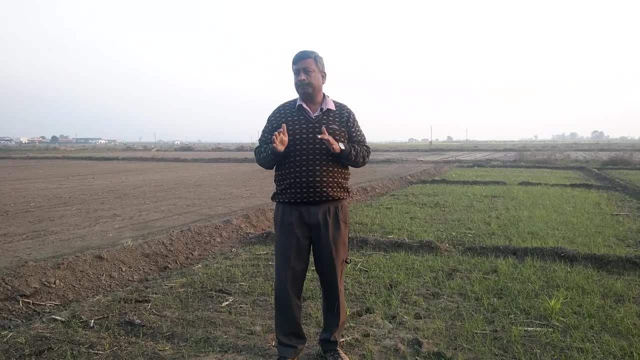 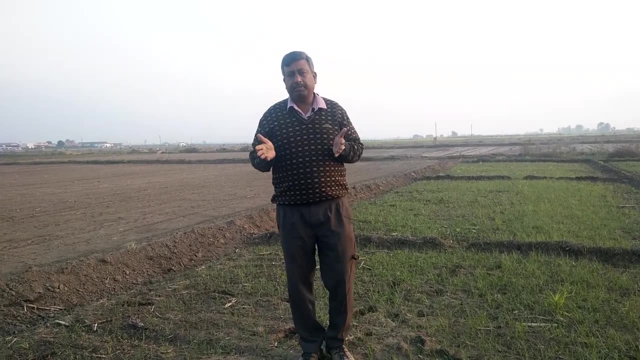 So what we see now? during decomposition, humus formation will take place, So there will be a process. mineralization will also take place. immolation will also take place. So I told you how the nutrients are released during the decomposition. 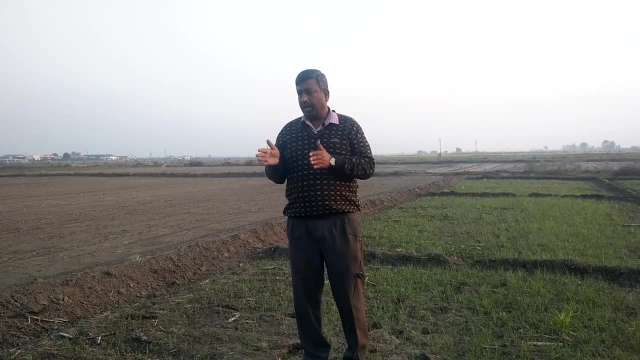 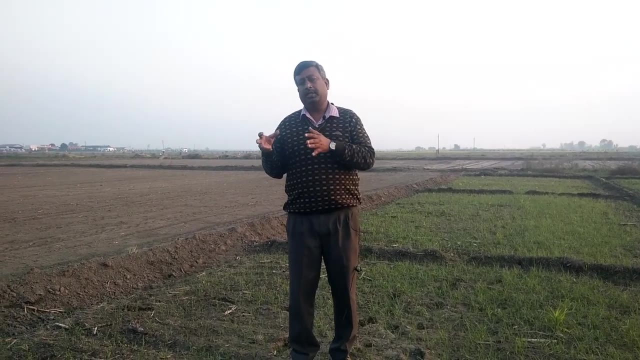 Now, it will depend on how the material is. If the material- see, this is the material. See, this is the material. If the material is more- see, if the cellulose hemicellulose is more, then what will happen? 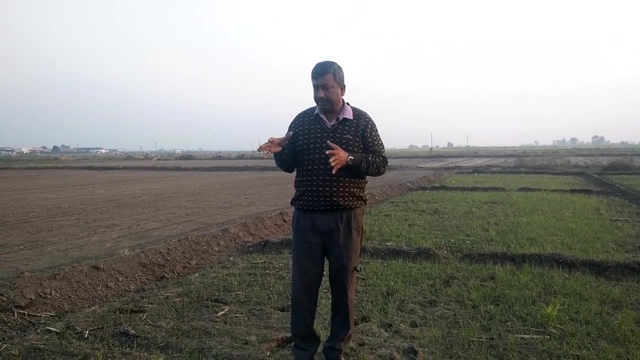 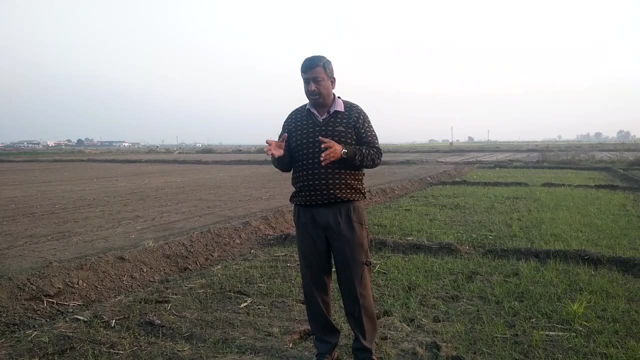 in that Decomposition will be very slow and nutrients will be released gradually. So this: I told you how this process will be done. Now see what happens. CN ratio: there is a great importance of the carbon-nitrogen ratio. 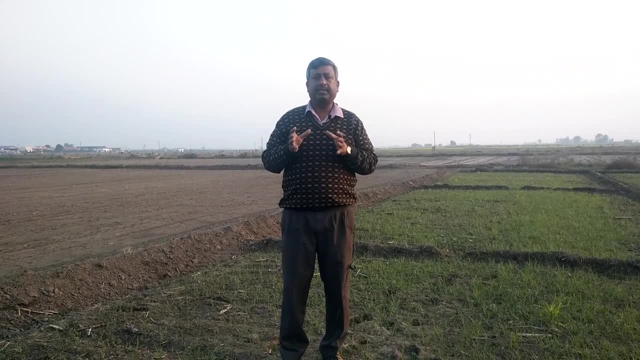 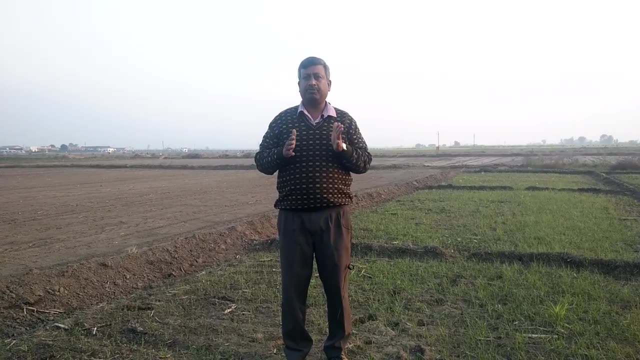 So in general the CN ratio in the soil is 10 to 12 to 1.. So the organic matter: it contains about 60% organic carbon and about 5% organic nitrogen- organic nitrogen and 60% about organic carbon. so the ratio is 12 to 1,. so in one soil the 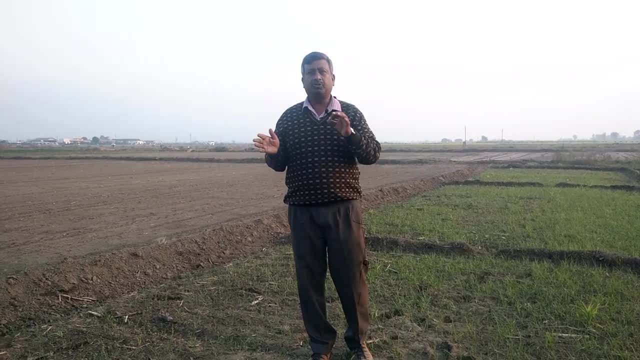 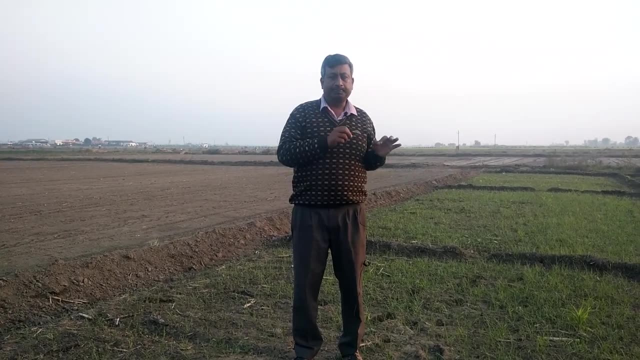 ratio is 10 to 1 to 12 to 1, so if we look at the carbon atoms, if 10 atoms are of carbon, then one atom will be of nitrogen. that is 10 to 1, if we are saying 12 to 1, then 12. 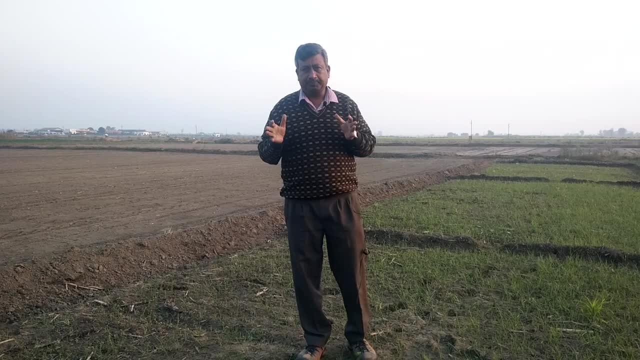 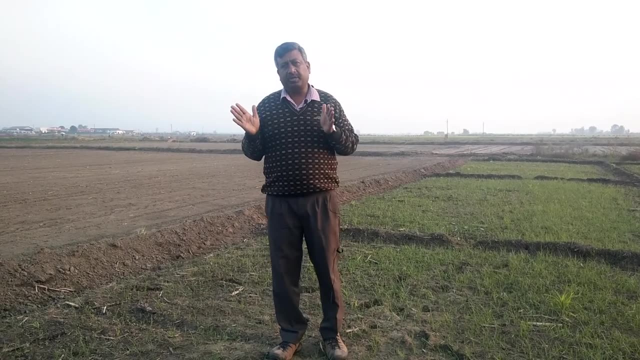 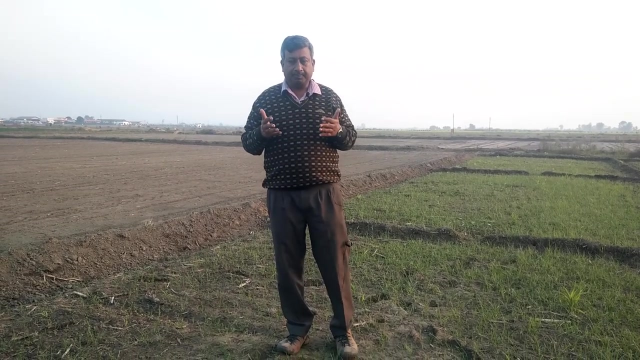 atoms are of carbon, then one atom will be of nitrogen. this is CN ratio and in soil. so the ratio of any soil is fixed. if we increase or decrease the organometer, then over a period it will become constant. Now what happens is that during the decomposition, microbes need both carbon and nitrogen. why? 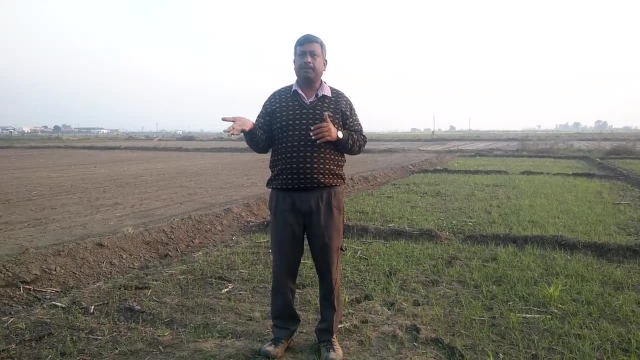 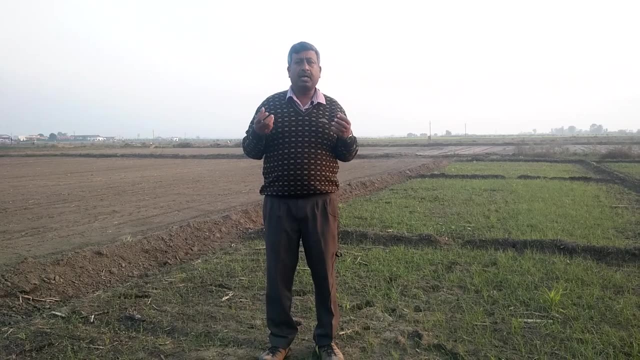 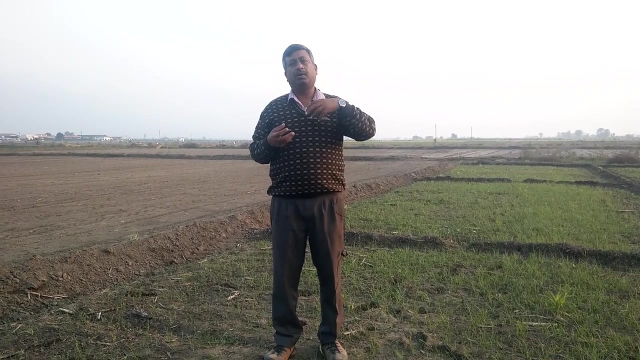 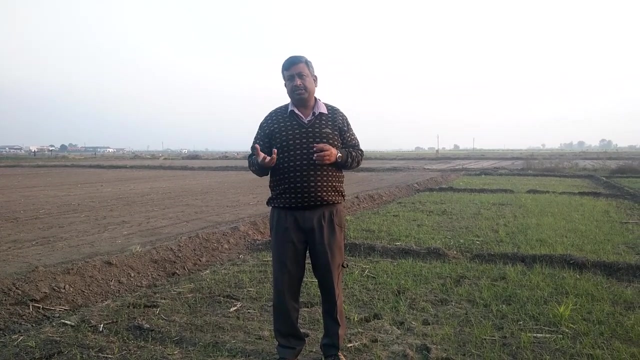 do we need carbon For cell synthesis and why do we need nitrogen For protoplasm? so when microbes decompose, they consume both things, carbon as well as nitrogen. So what happens with carbon? It becomes an exhaust. After cell synthesis, respiration will happen and it will go to CO2, nitrogen will come to its body and even after the body, the microbes will be mineralized and the soil will be a solution. 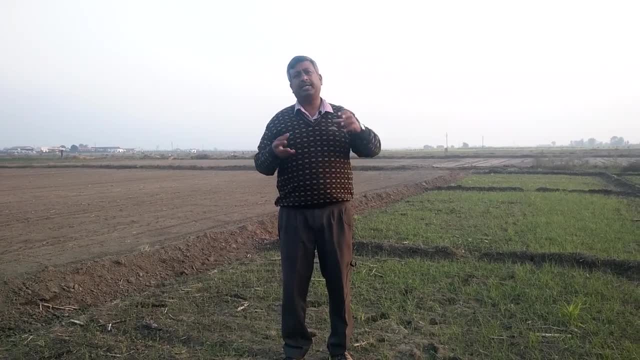 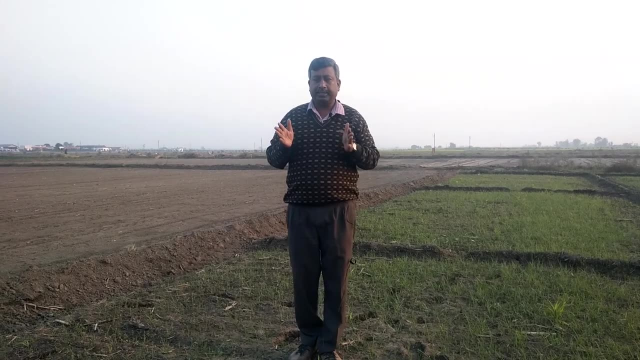 So slowly in the form of carbon dioxide. the carbon will go away, but the nitrogen will remain in the soil, So the CN ratio becomes narrow. So if we look at the CN ratio of microbes, the bacteria's CN ratio is 4 to 1.. So this means that if four atoms are needed for carbon, then one atom is needed for nitrogen, because if there is more protein in it, then more is needed for nitrogen. Fungus has a CN ratio of 9 to 1.. So the fungus has a wide CN ratio of 9 to 1.. 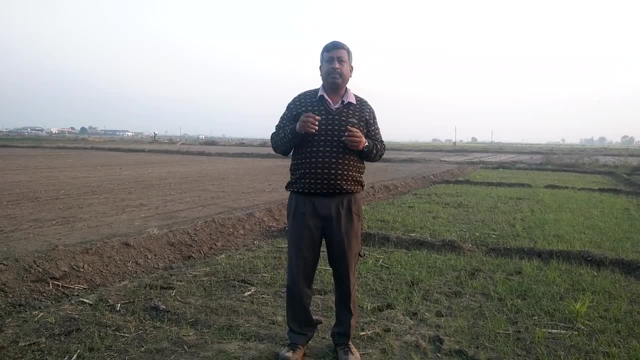 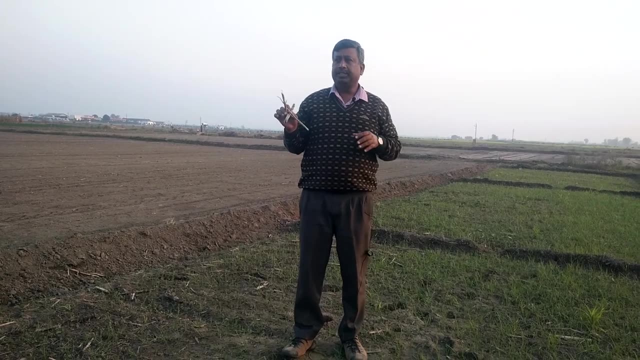 Fungus does not need so much protein. Now look at the CN ratio of the plant material. If we look at the CN ratio of these straws, it is about 100 to 1.. So this is for maize or wheat. They are around 100 to 1.. 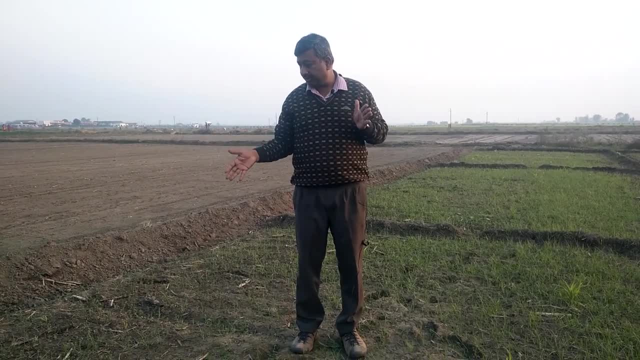 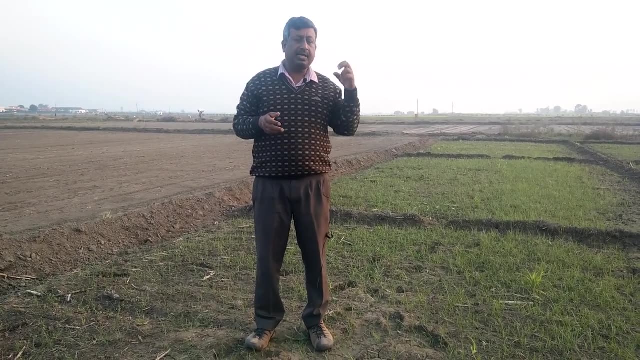 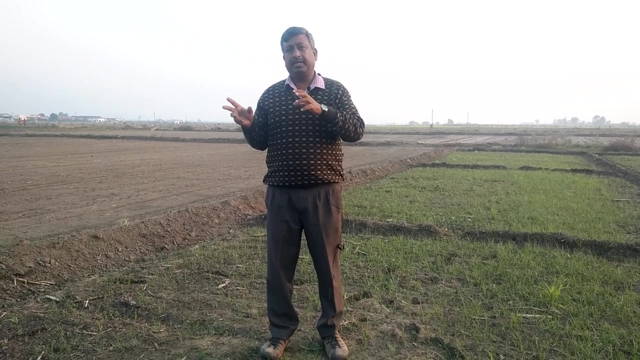 So now see how much is needed for microbes: 4 to 1.. And how much residue did we put 100 to 1.. 4 to 1 means that the bacteria needs one atom of nitrogen with four carbons. But in this, with 100 carbons, what we are taking, we are getting only one nitrogen. 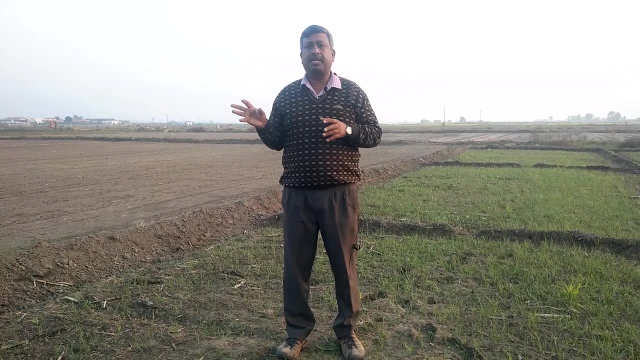 So this means that if the bacteria is attacking it, then what is nitrogen in it? It is deficiency. If the bacteria attacks it, then it is deficiency. So if the bacteria attacks it, then it is deficiency. Now, in this case, the reason of the problem is that the nitrogen is taking more out of the soil. Now, in this case, if the bacteria attacks it, then what is nitrogen in it? They are taking 100 carbon. Accordingly, they want more nitrogen. but in this, what is nitrogen? It is less. So, in case of such a case, what the bacteria will do? 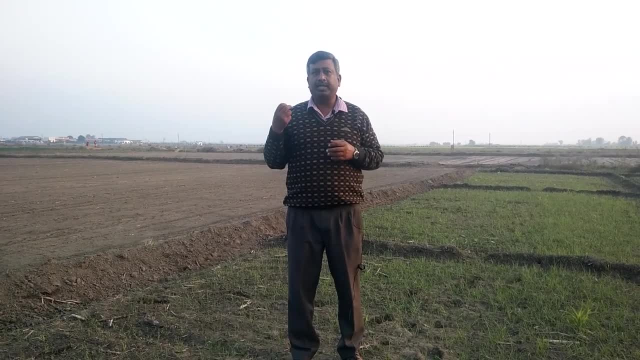 The nitrogen of the soil solution will also take, and it will take its own nitrogen will also take. the nitrogen of the soil solution will also take the nitrogen of the soil. So what will happen? in the soil Deficiency will come. this is immobilization. Now, if we put a residue whose CN ratio is very wide, then what will happen? The population of the bacteria will increase. from where will it take the most of the nitrogen? It will take from the soil solution. Now, if we put a residue whose CN ratio is very wide, then the population of bacteria will increase and the maximum nitrogen will be taken from the soil solution. 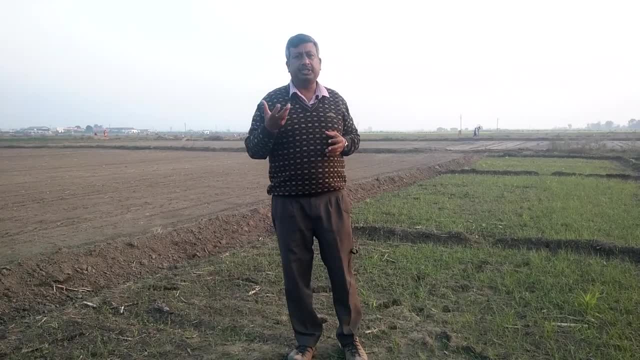 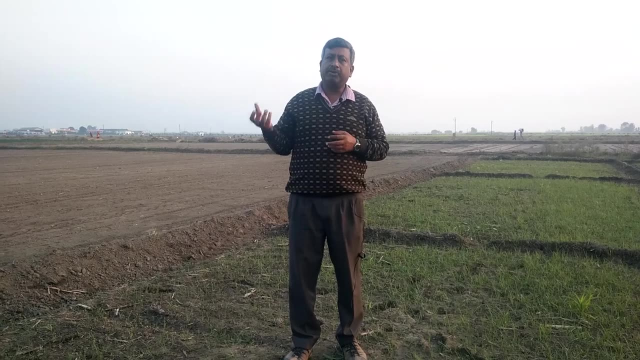 And if we put such a residue like legume- legume has about 30 to 1, then what is in it? If the nitrogen is good with carbon, then it will not take that much nitrogen from the soil because the legume residue is fulfilling it. So this will depend on the residue that how many microbes are taking from the soil solution. If we have put a residue with a very wide CN ratio, then the bacteria will take it from the soil solution and there will be a temporary deficiency. It is not that nitrogen has gone away from the soil. actually the nitrogen was locked in the bacterial cell. So this is temporary nitrogen deficiency and this is due to immobilization. So it is also known as nitrate depression period And it is in general 4 to 8 weeks. 4 to 8 weeks means it can be 1 to 2 months. 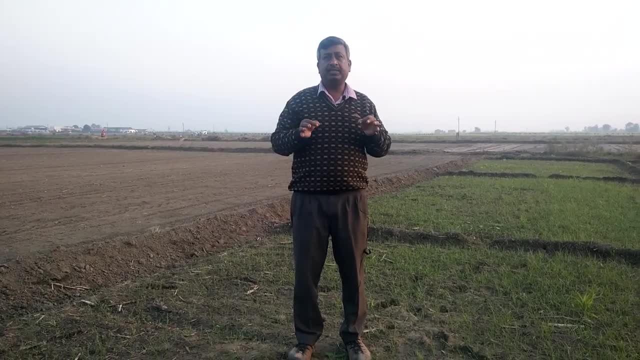 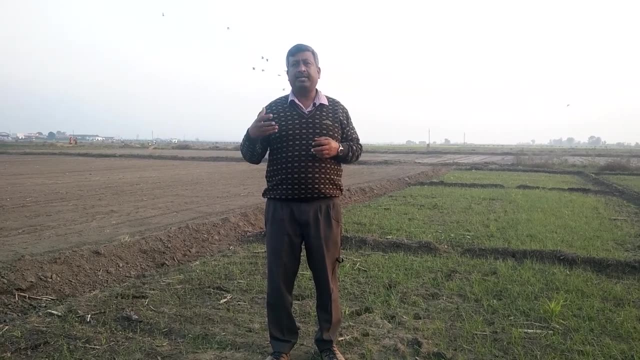 But it will depend on the material. Remember this: If there is a good CN ratio, then it will decompose very quickly. If there is rice or wheat or maize, then it will decompose slowly. Nitrate depression period will be more in it. 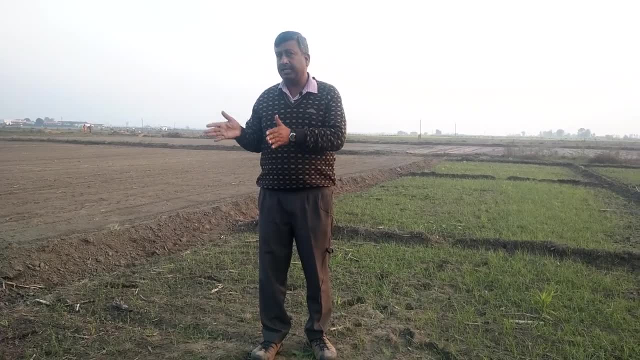 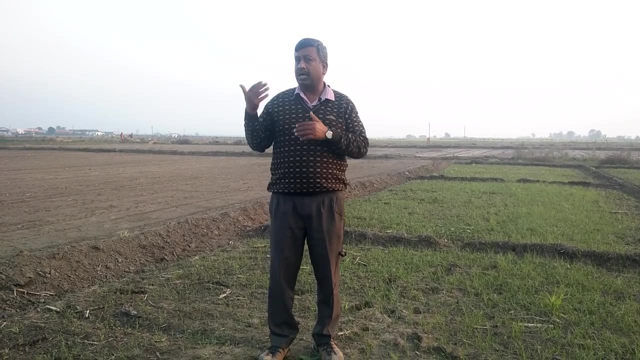 So whenever we mix the residue, it means that if the crop is sown after mixing the residue, then there will be a deficiency of nitrogen Because the bacteria will take that nitrogen Because it got the carbon but it did not get the nitrogen from the residue. 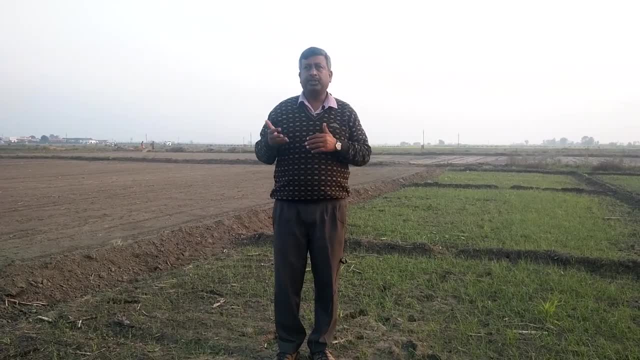 So where did it take the nitrogen from? It took it from the soil solution. So this deficiency came. So whenever we mix the residue we should be careful. We should know that we incorporate the residue about a month ago, One or two months ago. 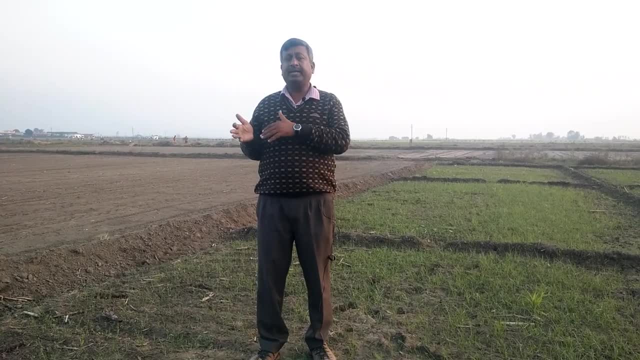 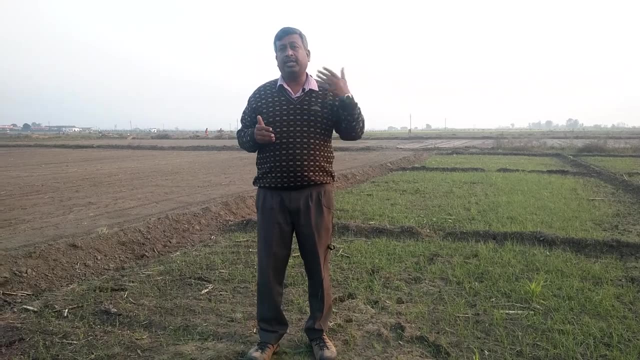 If this is not possible, that we are not able to incorporate the residue one or two months ago. We have to incorporate the residue and we have to sow it immediately. Then what should we do? We will add extra nitrogen from outside. We will add urea. So that who gets the nitrogen? The bacteria will get it And the requirement of their body will be fulfilled And they will not take nitrogen from the soil solution. Now what will happen When they will take the nitrogen? their death will happen and it will be released. 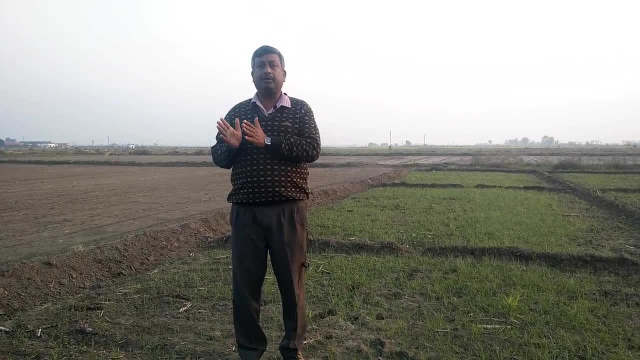 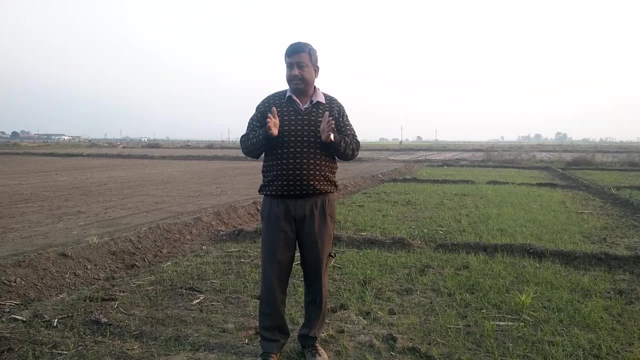 So it is not that there is a loss of nitrogen. This is temporary locking. Temporary depression or temporary deficiency of nitrogen comes. So this is the significance of CN ratio. How does CN ratio decide Crop residue or whatever organic matter we are adding? 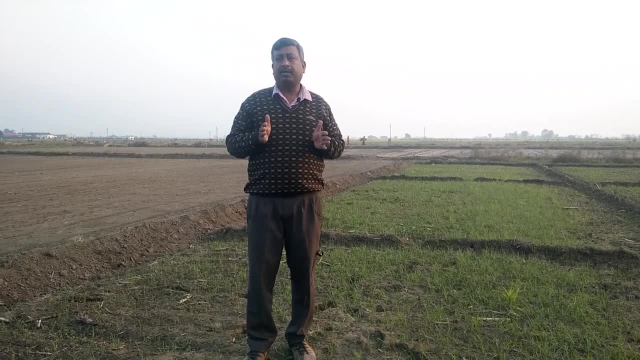 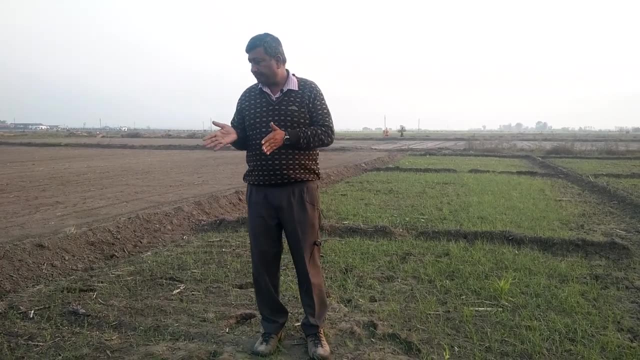 If there is a narrow CN ratio, then it is very good. If there is a wide CN ratio, then what will happen? There will be a deficiency of nitrogen, So this affects the rate of decomposition. If there is a residue with a wide CN ratio, then there will be a very slow decomposition. 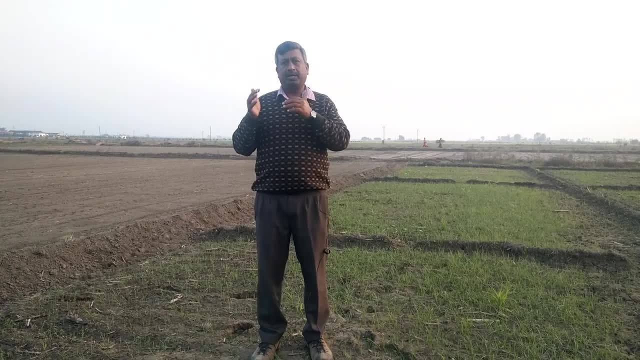 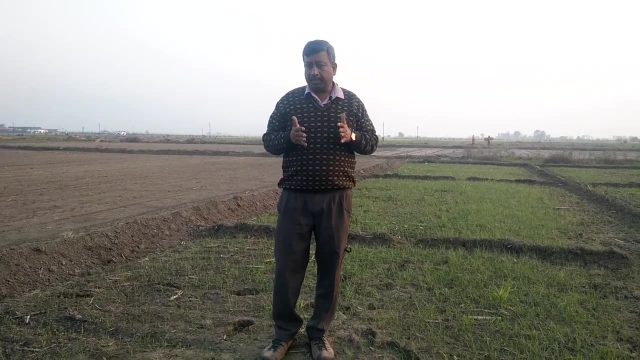 and the nitrate depression period will be more. If there is a residue with a narrow CN ratio, then the decomposition will be very fast and the nitrogen will be mineralized very quickly. So now we have to see whether the nitrogen will be mineralized. 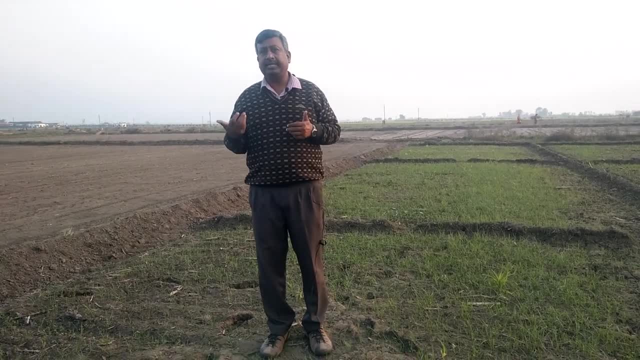 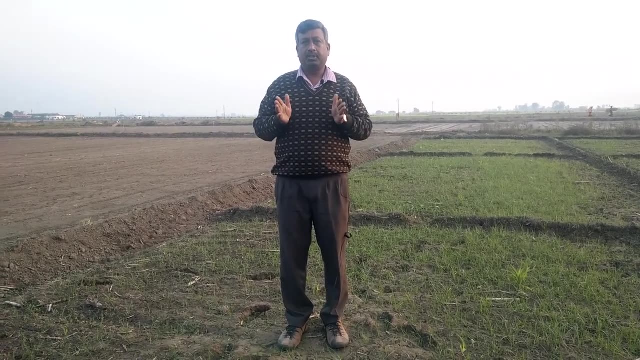 that is, it will come in the soil solution or it will be immobilized. it will go to the bacterial cell. It depends on CN ratio. So if the CN ratio is less than 20 to 1, then nitrogen will be mineralized. 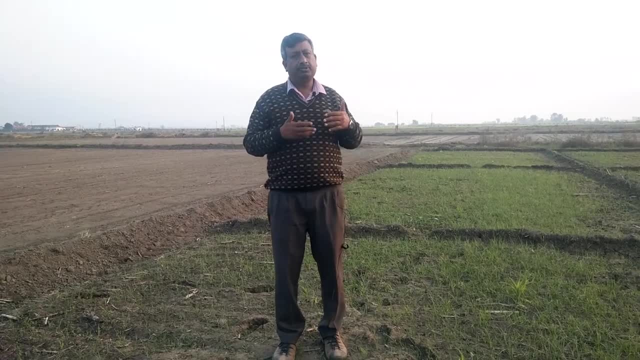 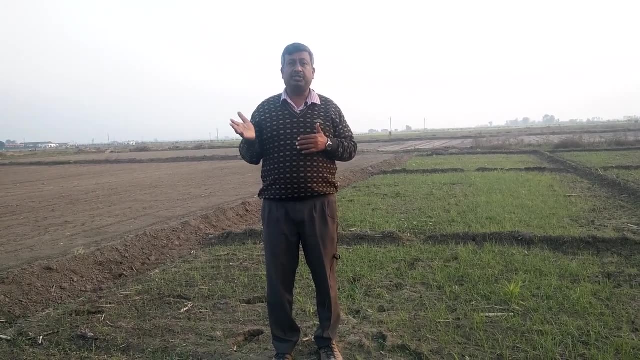 In such a case, the nitrogen requirement of the bacteria will be fulfilled and the nitrogen will remain in the soil solution If it is more than 30 to 1, if the CN ratio is more than 30 to 1, if the CN ratio is 30 to 1 in this residue. 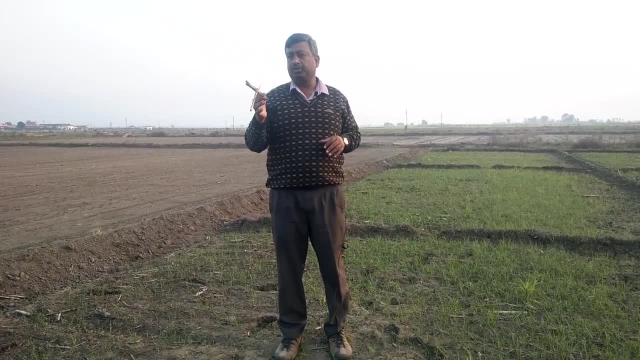 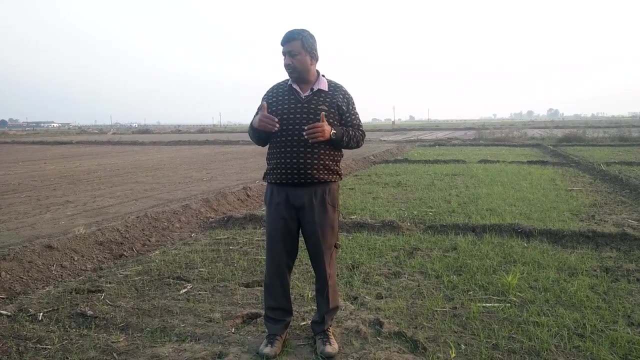 then nitrogen will be immobilized. So look, the residue of maize has a CN ratio of 80 to 90 to 1. So when the residue of maize is found, it means that here the nitrogen will be immobilized and it will be released after about one and a half months. So if it is less than 20 to 1, then it will be mineralized, and if it is more than 30 to 1, then it will be immobilized. Now let's talk about if it is in between these two, if it is between 20 to 30 to 1,. 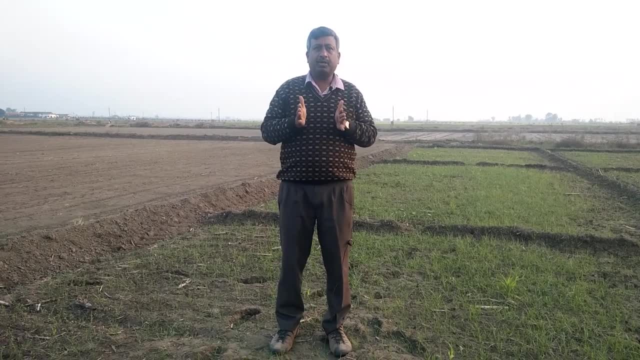 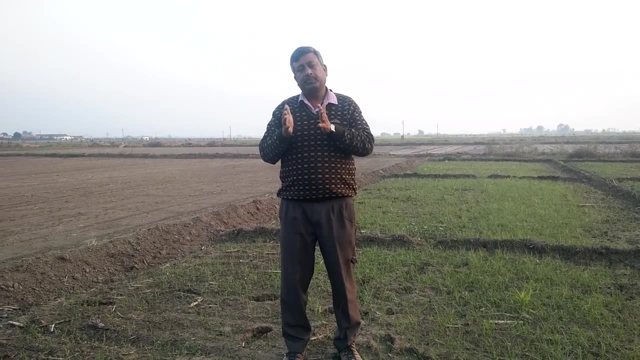 if it is more than 20 but less than 30, then in such cases what happens is that it is a little mineralized and a little immobilized. So in this whole process we can say that neither it will be immobilized nor it will be mineralized. 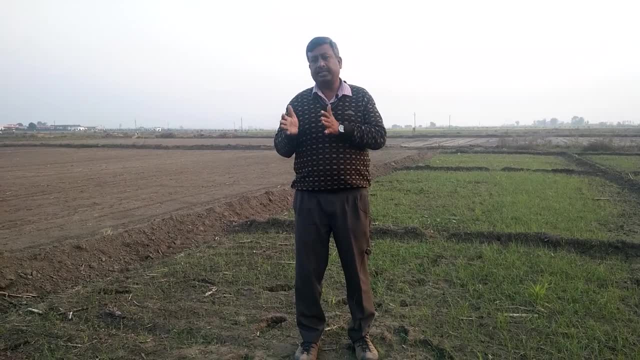 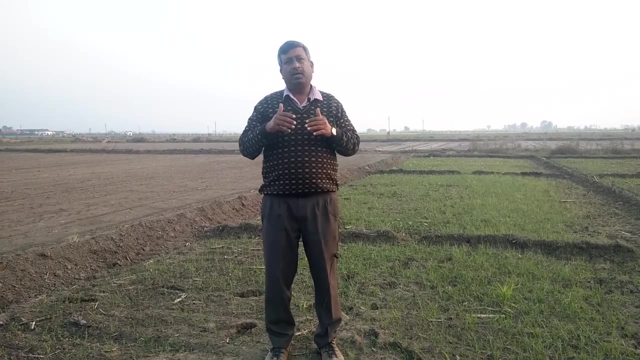 The total net mineralization is. and if we see the net mineralization, then what will happen is that both will be equal. So in such cases, neither the proper plant will get it, nor will it go properly to the microcell. What will remain between the two? 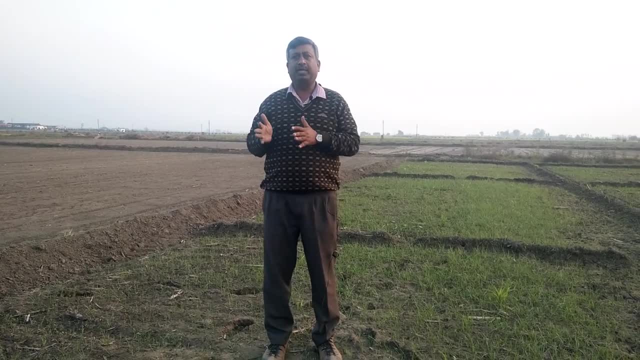 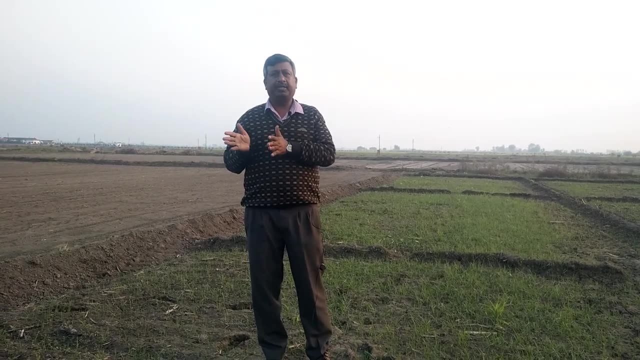 The net balance will remain zero. So if we get a residue, whether it is a weed residue, whether it is a straw or any other residue, either we give a waiting period for nitrate depression period. if we do not have a waiting period, 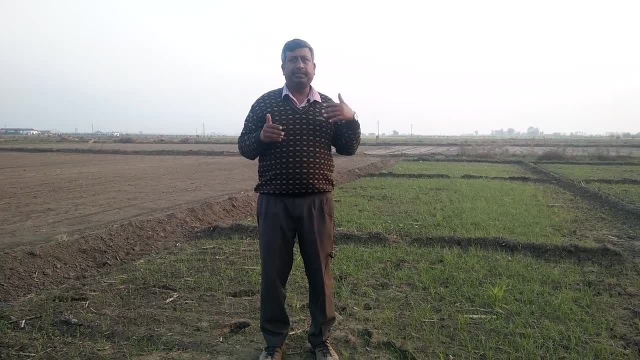 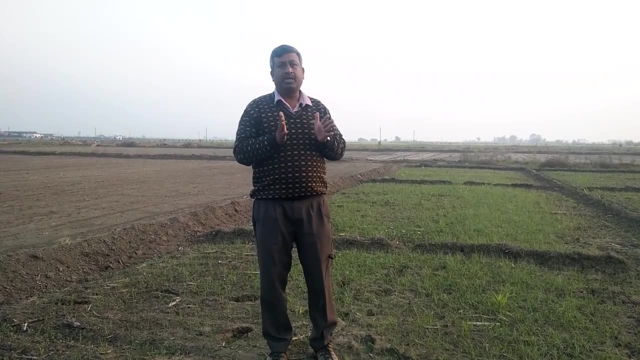 then we give a little external nitrogen source in it so that it decomposes quickly. Now for green manuring we use sasban or dhencha. So see in dhencha what is the CN ratio. already CN ratio is very narrow. 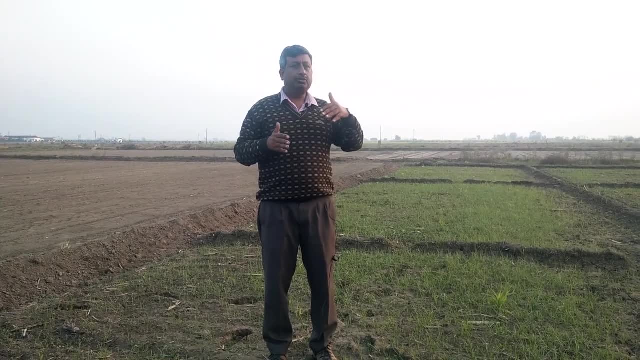 I told you about legume. It is about 20 to 30 to 1.. So if the CN ratio is less than 20 to 1, then what happens is that it decomposes immediately. That means the microcell attack is fast in it.